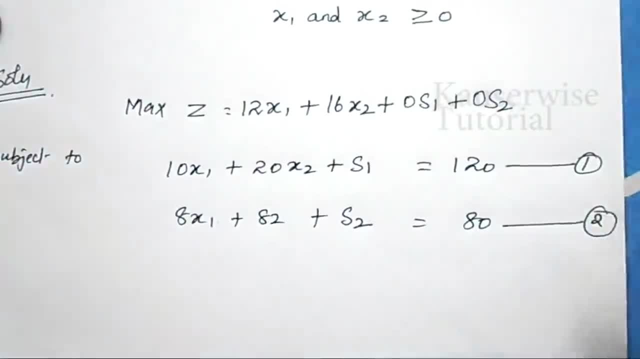 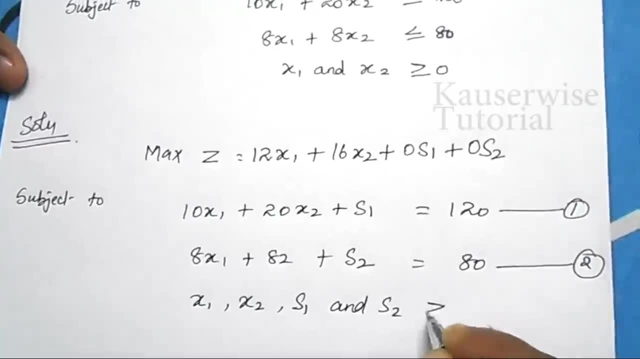 This one is first constraint and this one is second constraint. So x1 comma, x2 comma, s1 and s2 greater than 0. This should be equal to 120.. Let us see how I am going to figure out how girls to get проблемы with the this, this and this. 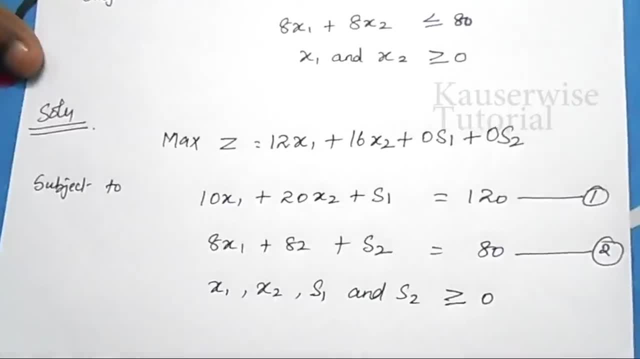 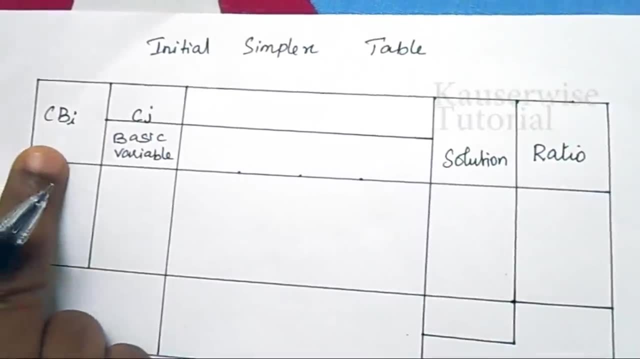 We know that every girl should be able to get problems in A and B. that is the way I am To know the reason for the strength of all our children. I will tell you the reason in the frame, the initial feasible table: see. this is the format of initial simplex table: see. here cbi is. 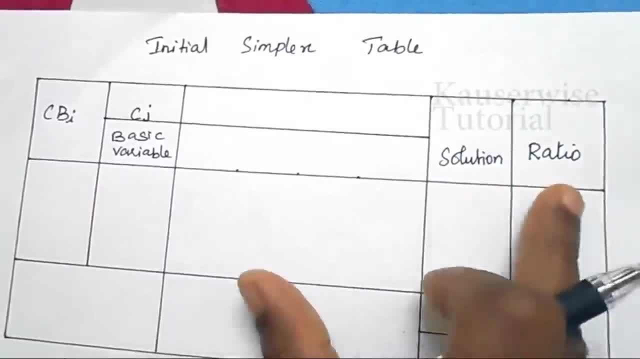 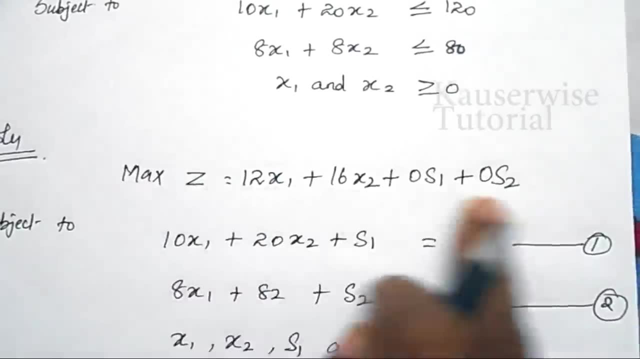 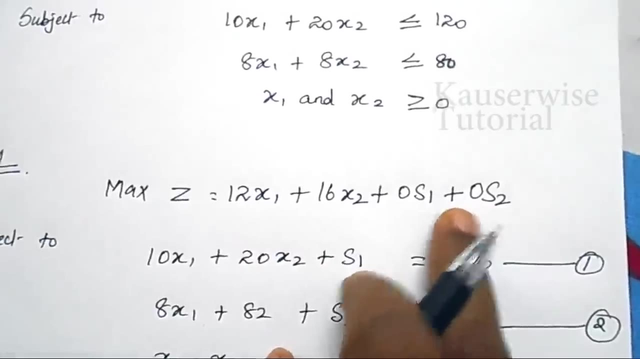 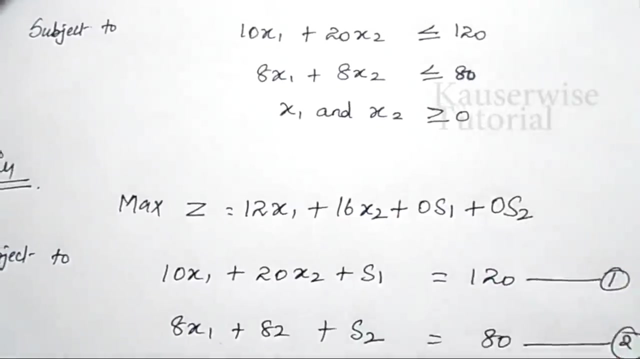 the cj basic variables solution. this column for ratio cj refers to coefficient of the objective function. so coefficient of objective function is for x1 12, for x2 16, for s1: 0, for s2: 0. so these are the coefficient of objective function. so you need to write these values in this column. cj is: 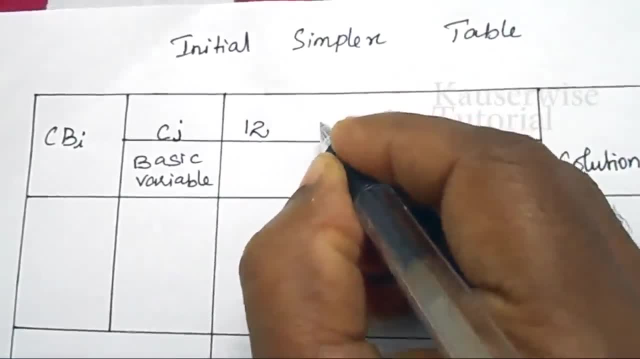 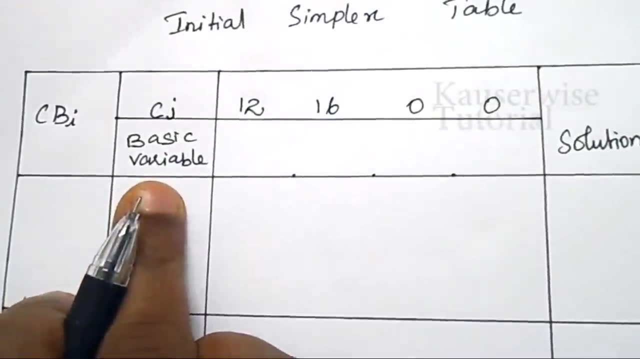 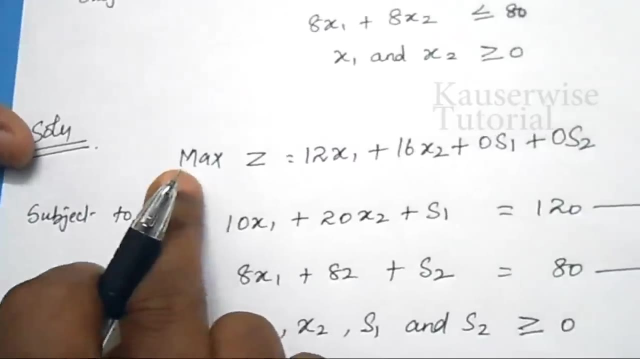 12, x1, 16, x2, 0, s1, 0, s2. so we have four basic variables now: x1, x2, s1 and s2. again see the objective function. 12 x1 cj is coefficient. is 12 x1, 16, x2, 0, s1, 0, s2. so we have four basic variables now: x1, x2, s1 and s2. again see the. 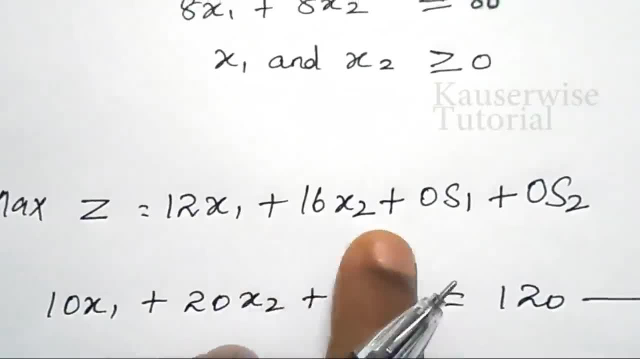 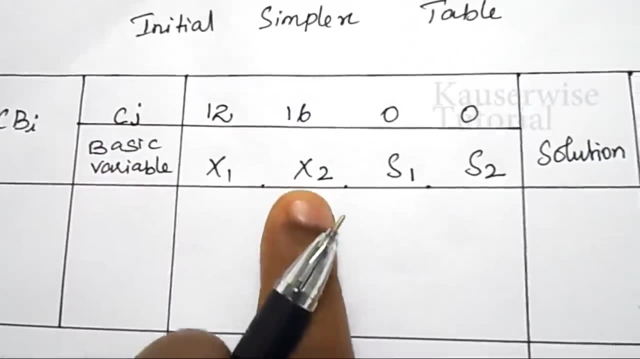 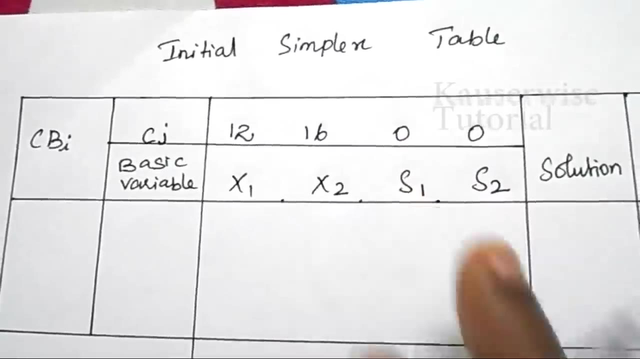 objective function: 12: x1. basic variable is x1, second one 16, x2. 16 is coefficient, x2 is basic variable. cj: 16: basic variable: x2. then 0, cj is 0. basic variable is s1, 0, s1. and the last one is: 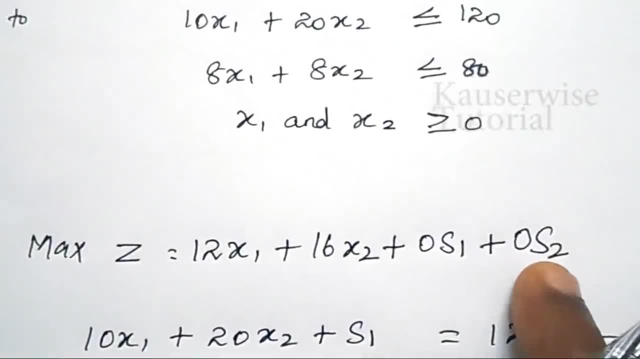 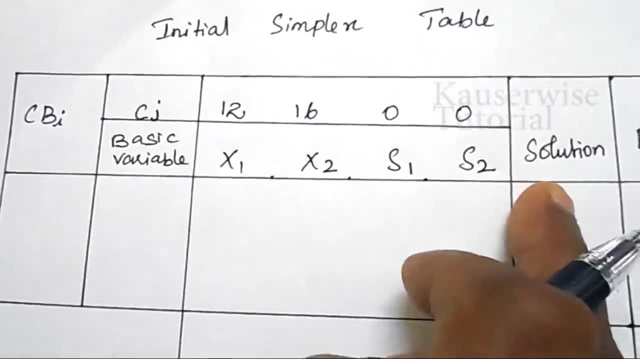 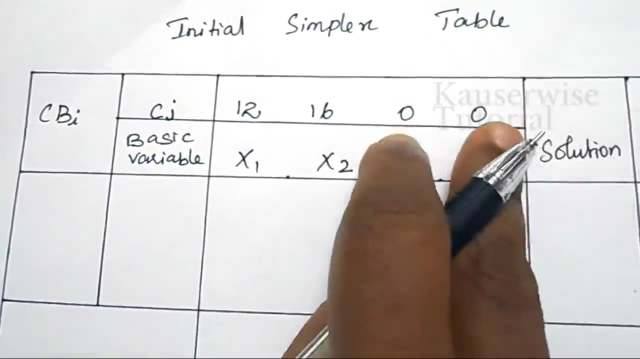 0 is cj and s2 is basic variable. 0 and s2, so these are all cjs and basic variables. so here cj is 0 and s2 is basic variable. so here cj is 0 and s2 is basic variable. so here in this objective function we have two basic variables. we have added two basic variables. 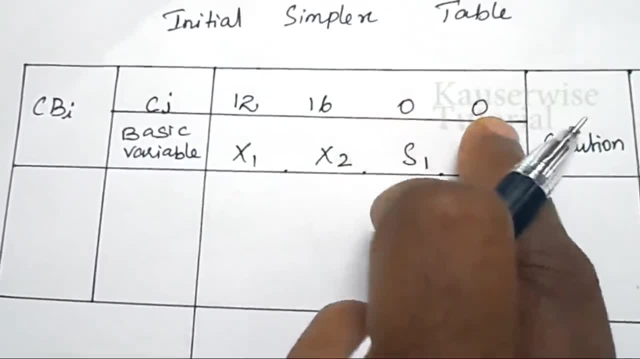 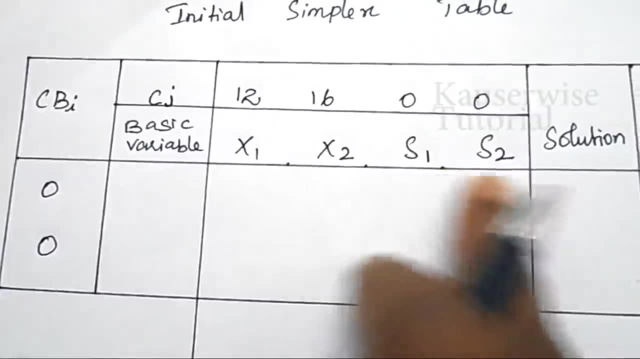 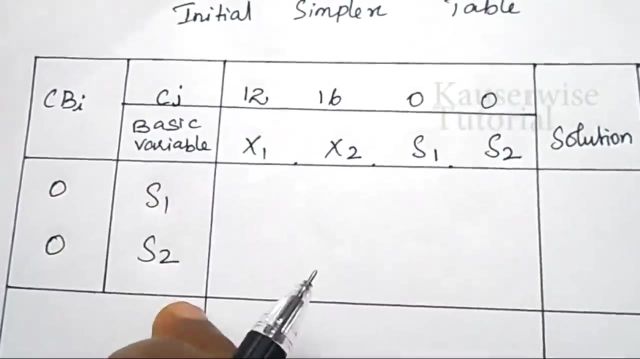 now what is the value of basic variable 0 and 0? here you need to write the values. that is coefficient of basic variable. so we have introduced two slack variable now. so here you need to write s1 and s2. so these are the two slack variable which is called as basic variable. look at the 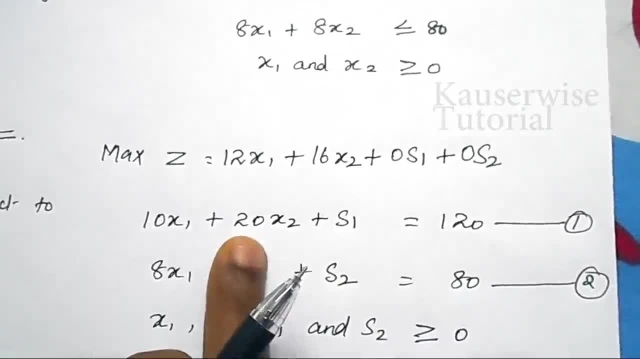 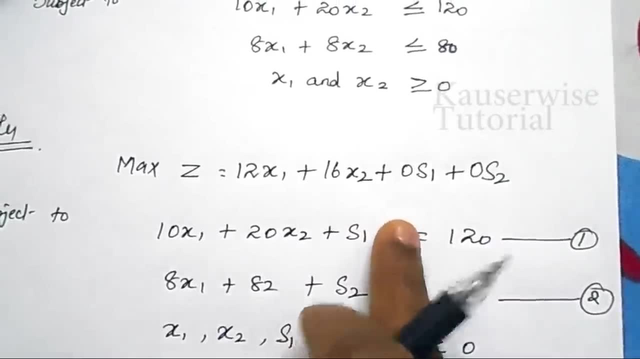 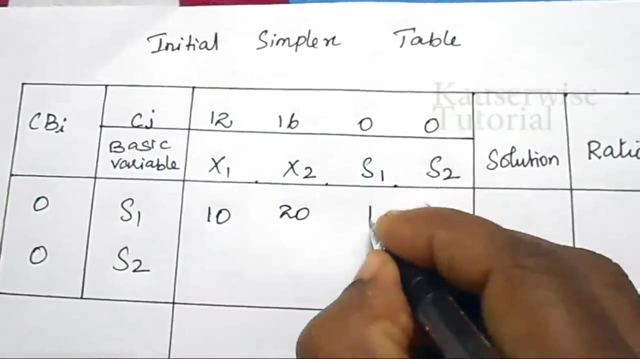 first constraint: 10 x1 plus 20 x2, plus only one slack variable introduced in the first constraint, so 1 s1, no s2. so for that you can put: 0 is equal to 120, 10 x1, 20 x2. only one s1 is there now in the first constraint, so no s2 in. 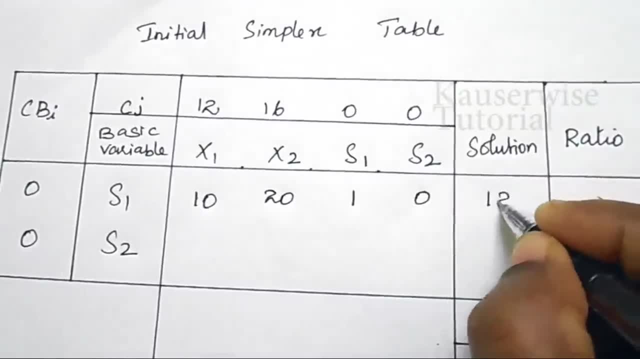 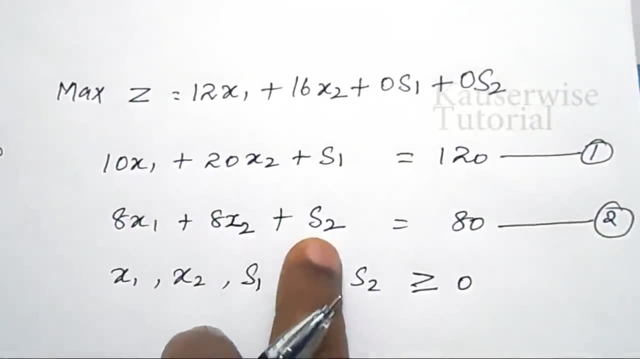 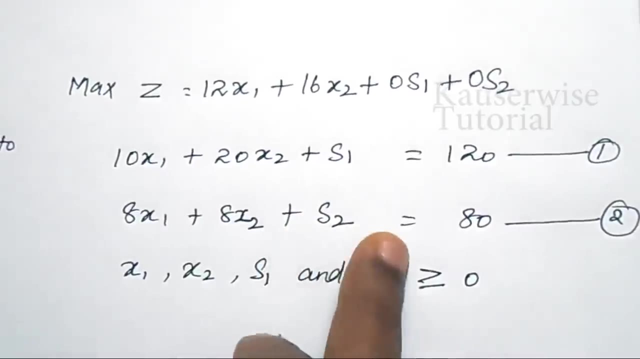 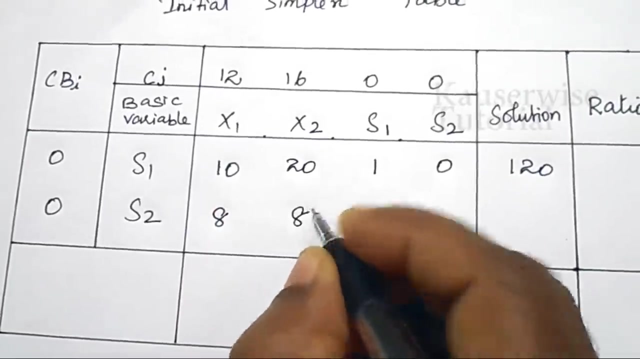 the first constraint is equal to what is the value? solution is 120. now look at the second constraint: 8 x1 plus 8, x2 plus s2. here no s1, here we have introduced s2, and s2 is the first constraint, s2. so s2 value is 1, s1 value is 0, is equal to 80. for second one: 8 x1, 8 x2, s1 value 0, s2 value is 1. 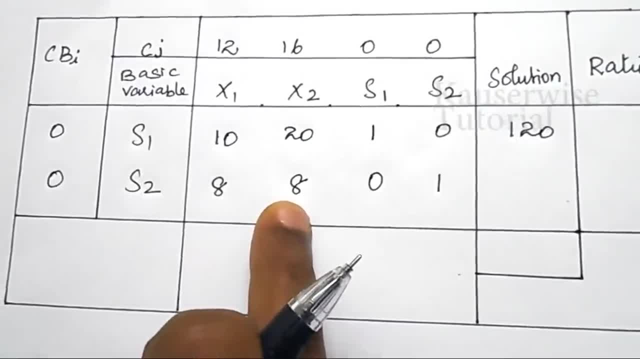 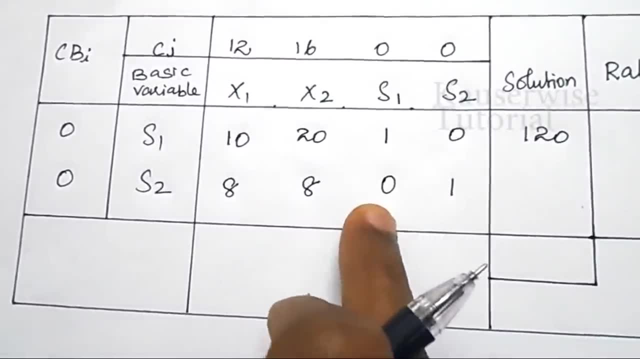 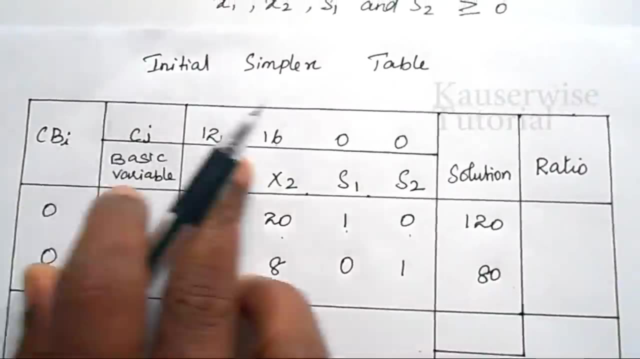 8, x1 plus 8, x2 plus s2. so here we have only s2, no s1. no, so for s1 you can put 0, we have s2, so put 1. let me explain the initial simplex table here: cj basic variables: are there? no, just look at the. 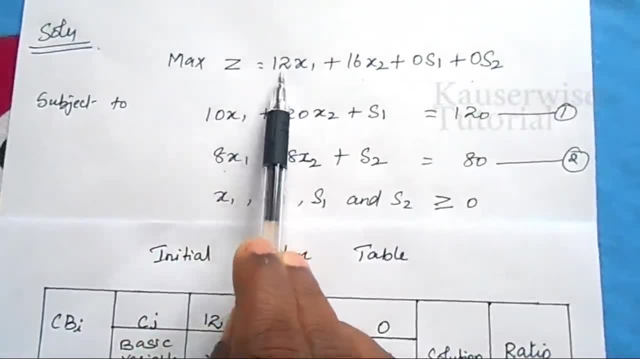 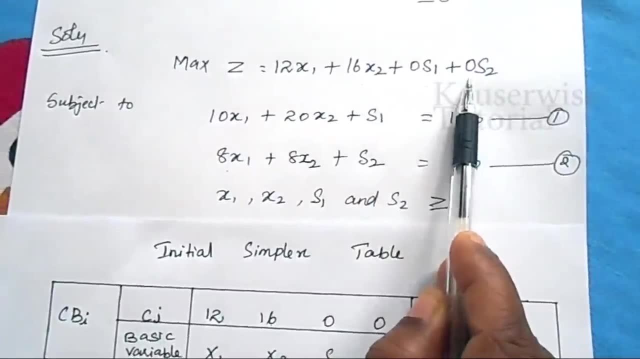 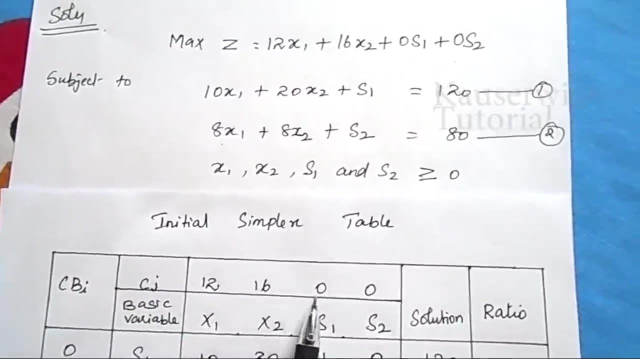 objective function maximization z is equal to 12, x1, 16, x2, 0, s1, 0, s2. no 12, 16, 0, 0s are objective functions coefficient: see cj refers to coefficient of objective function: 12, 16, 0 and 0 here x1, x2, s1. 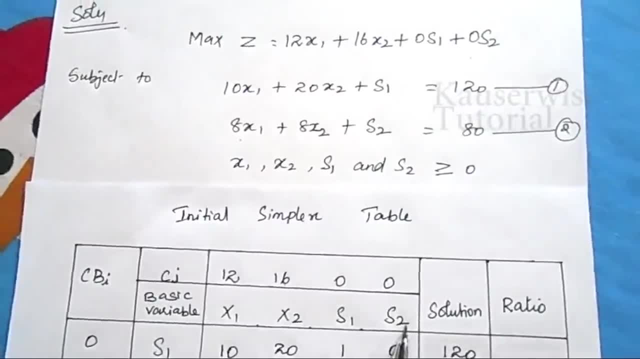 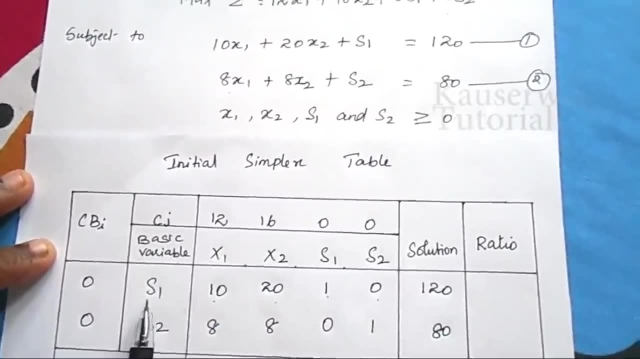 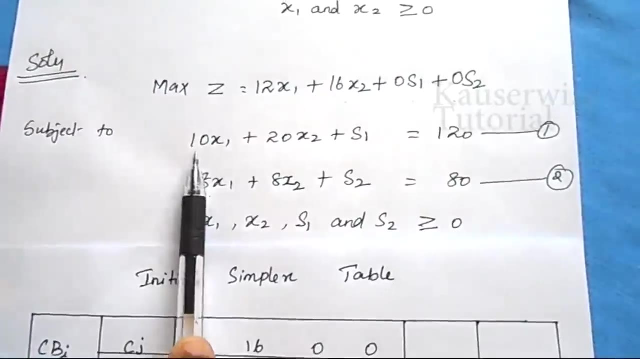 x1, x2, s1, s2. okay, so here in basic variables here we have introduced two slack variables, no, s1 and s2. for the first equation, s1 is a slack variable. for the second constraint, s2 is a slack variable. so look at the first constraint: 10 x1, 20, x2, no, 10, 20, here we have only one slack. 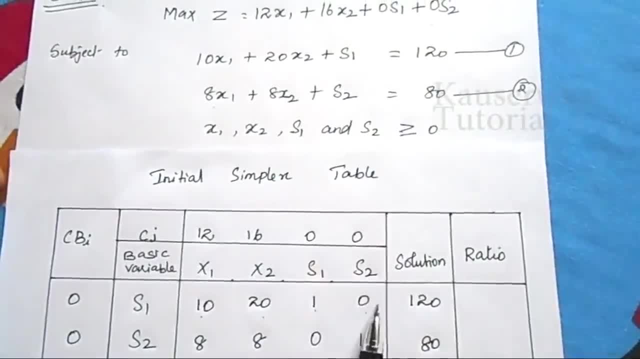 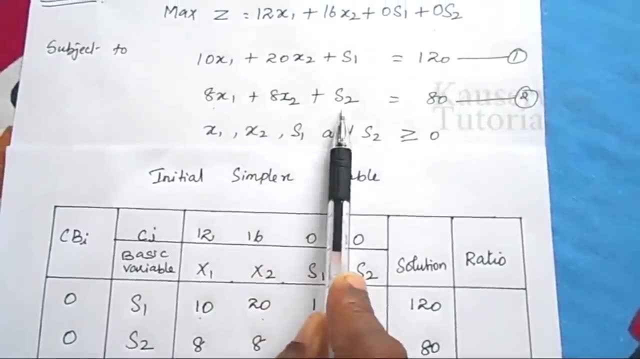 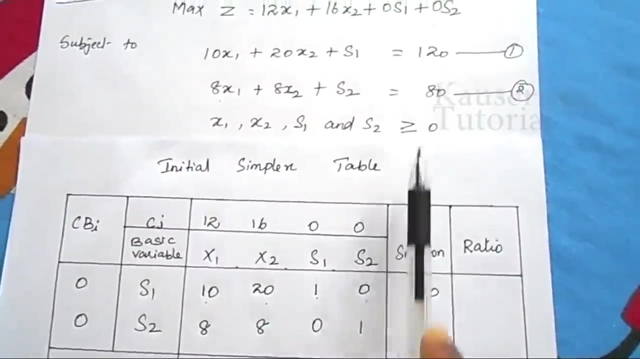 variable, that is s1 so 1, no s2 so 0, and 120 is a solution. look at the second constraint: 8 x1 plus 8 x2 and s2. okay, 8 x1, 8 x2, no s1 so 0. here we have s2, so 1. solution is 80. 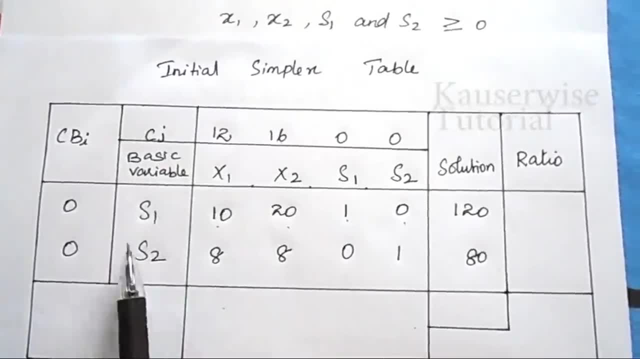 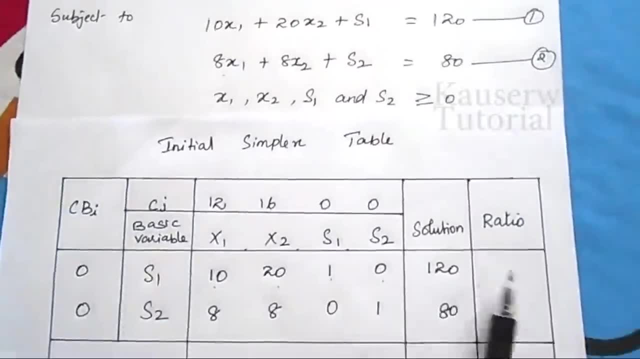 here we have two slack variables, no s1 and s2. the cost of slack variable is 0- 0. look at the objective function: 0 and 0. so this is the way to prepare the initial simplex table. now we need to find zj values. look at this formula. 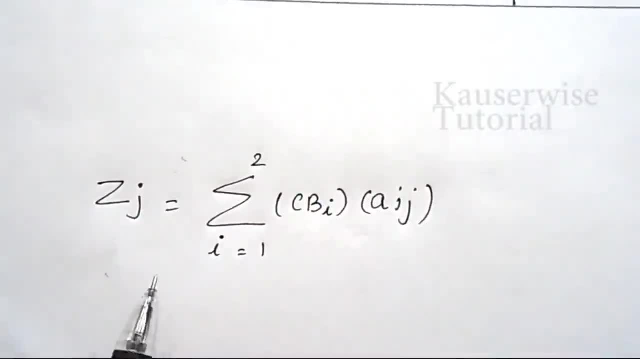 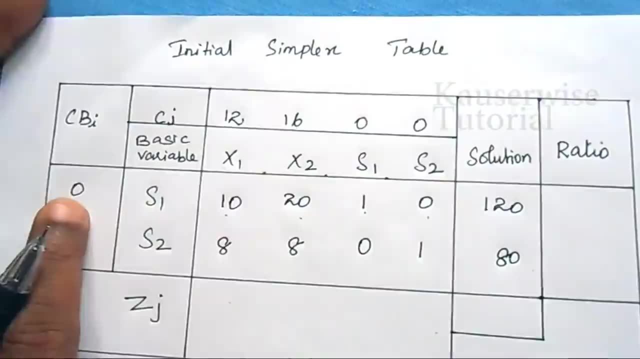 this is the formula to find the values for zj, but i am going to use a simple way to find out zj. see the first value: cbi into x1, that is, 0 into 10 plus 0 into 8. let me explain. first value is 0. 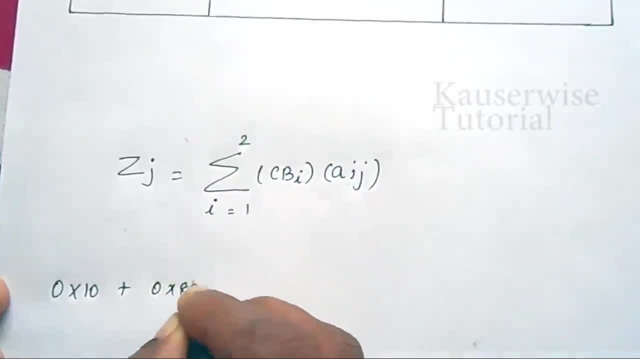 into 10 plus 0 into 8. so what is the value? 0 into 10 0 plus 0 into 8 0. so what is answer: 0 0 into 10 0, 0. so what is zj 0 into 10 0 and zj 0 into 10 0 cannot be created by the other way. 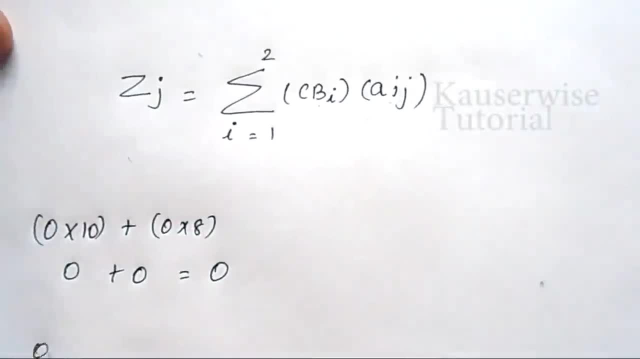 look at the third value: 1: 0 into 10 0 plus 5: 0 into 10: 0, so first variable is greater than 0. so no j isane for u. i am going to looking for something like n, as it will help you and the. 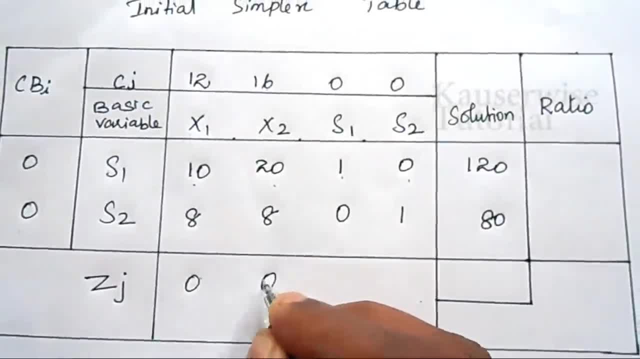 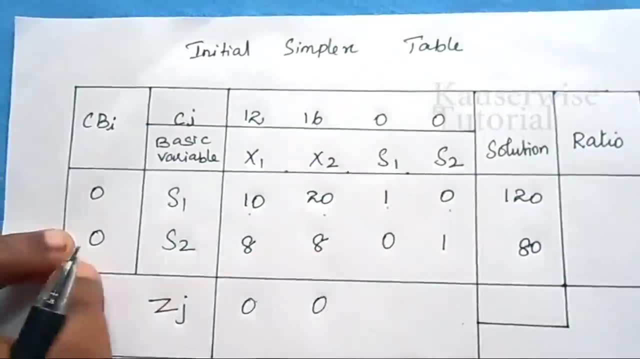 answer is okay. now let us look at the last variable. look at the second value: 0, 0 into 10 0 and zj 0. interesting answer: if you are going to achieve your zj maximum, in our case, again use a original alec To hacer Mathic. you have x2 right mark, z, y equal i. would be x1 plus 0 and z to that is zero in The second value, 0 into 20. x2 plus 0 into 8, 0, 0 into 10. x1, 0 plus 0 into 8: 0. explaining the future values, Look at the second value: zero into 20. 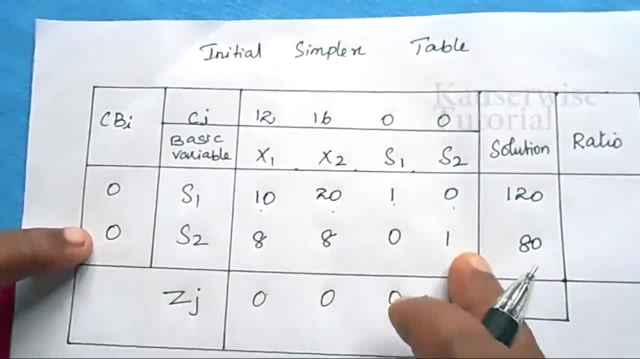 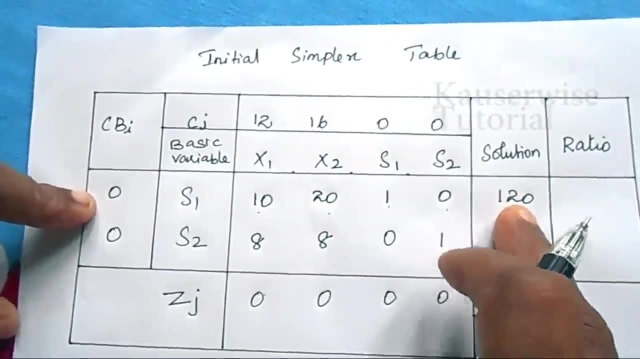 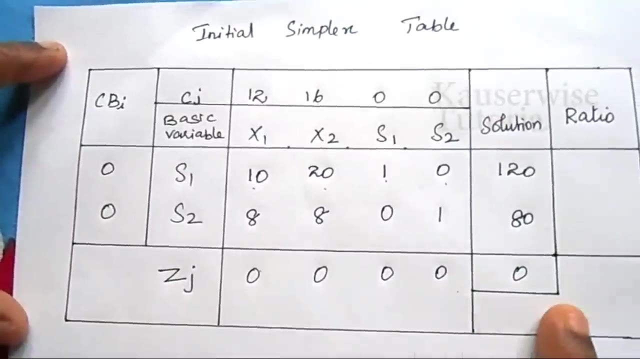 0 into 0 is 0 plus 0 into 1 is 0. value is 0. okay, the same way for the solution. also 0 into 120, 0 plus 0 into 80: 0, since our cbi value is 0. so all the zj values will be 0, only in the initial. 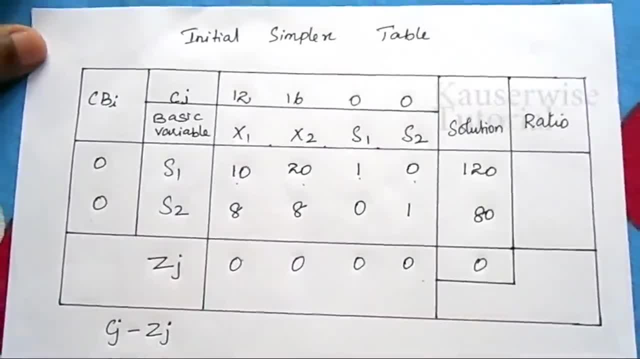 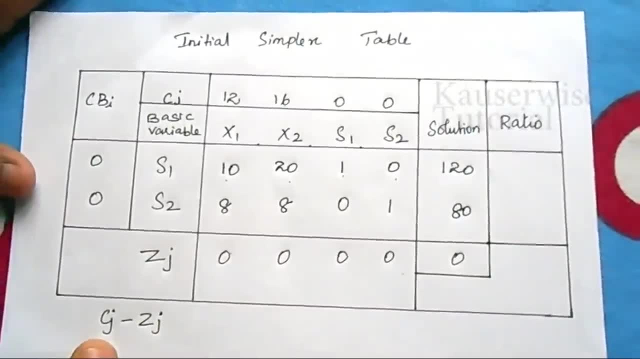 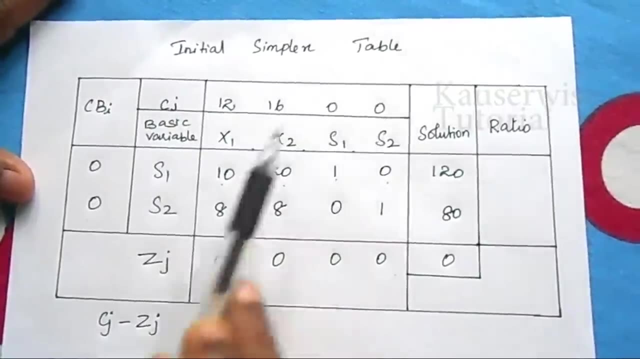 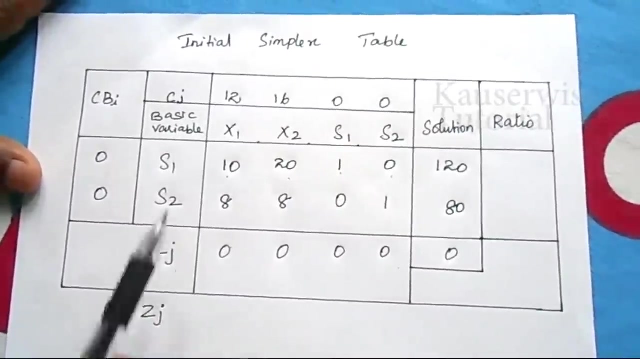 simplex table. after finding zj, now you need to compare cj and zj. the formula is cj minus zj, so cj is our coefficient of objective function. look at the top. cj is 12, 16, 0 and 0. zj values are 0, 0, 0, 0. just compare two values. that is cj minus zj. cj is 12, zj is 0, so 12 minus 0, 12. 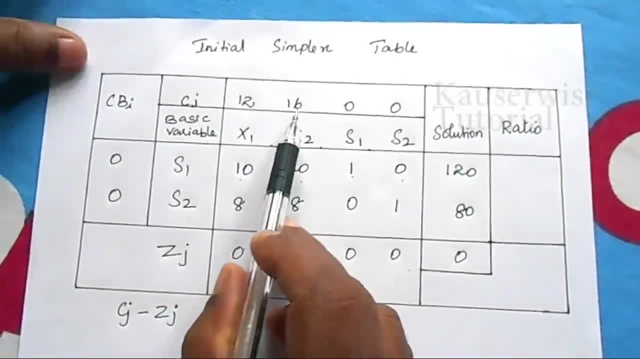 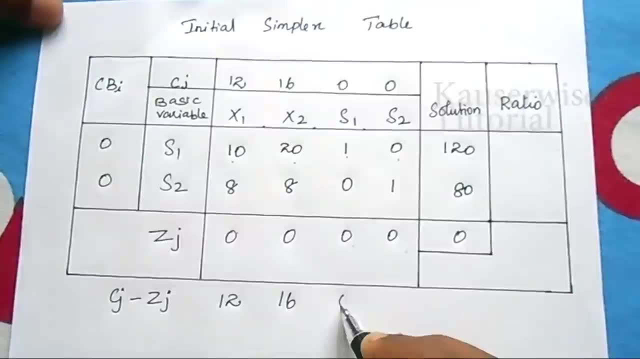 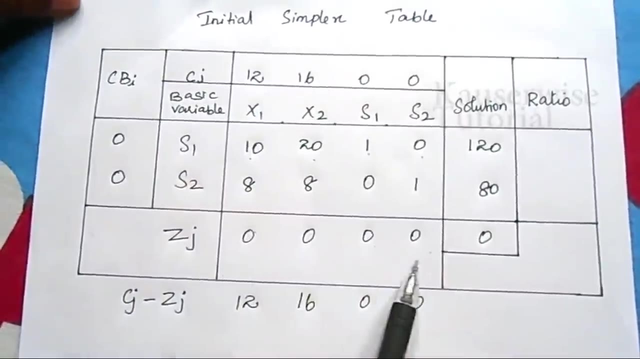 in the same way for the second value, cj value, 16 zj value is 0: 16 minus 0. 16. 0 minus 0, 0, 0 minus 0, 0. okay, so we have 4 cj values and 4 zj values and we have got these values. 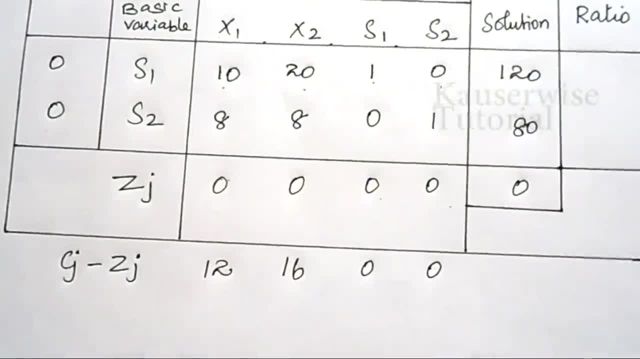 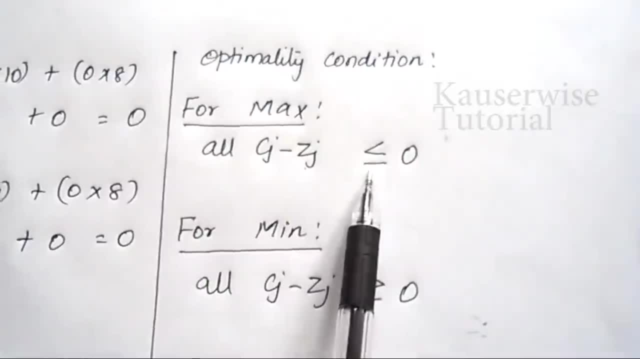 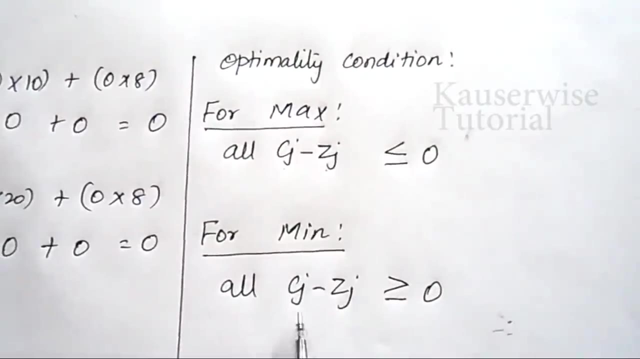 after finding cj minus zj values, look at the optimality condition. for maximization problem, all cj minus zj value should be less than or equal to 0, which means 0, or negative values. for minimization problem, all cj minus zj values should be greater than or equal to 0, which means 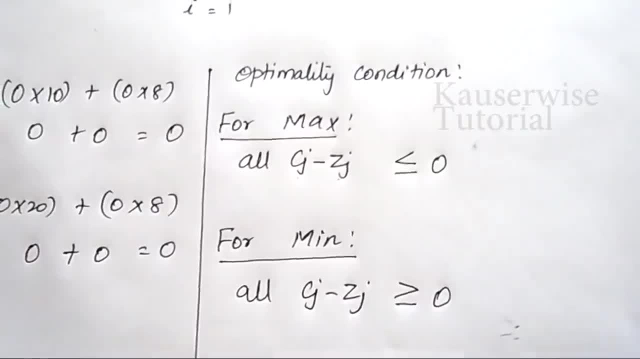 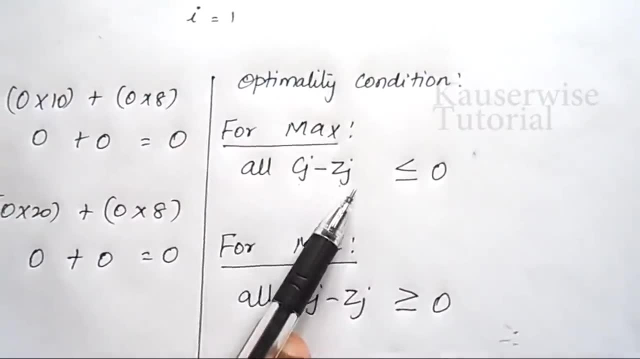 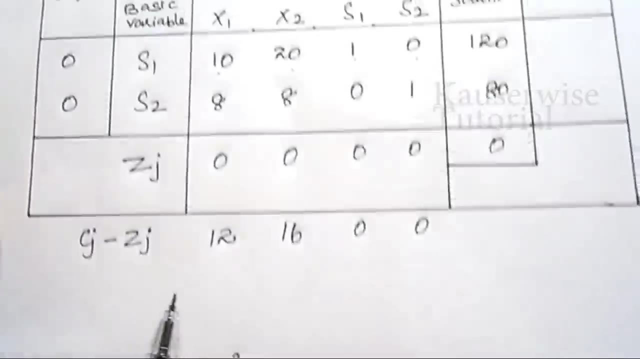 0 or positive values. so this is the optimality condition. so here this problem is a maximization problem. no, so our value, that is cj minus zj values, should be less than or equal to 0, which means 0 or negative values. but here we have got positive values. the first value is 12. second value: 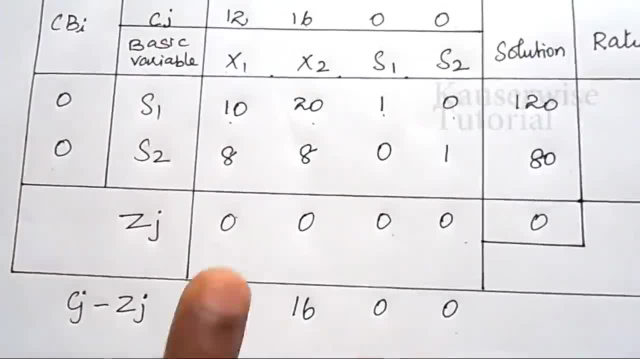 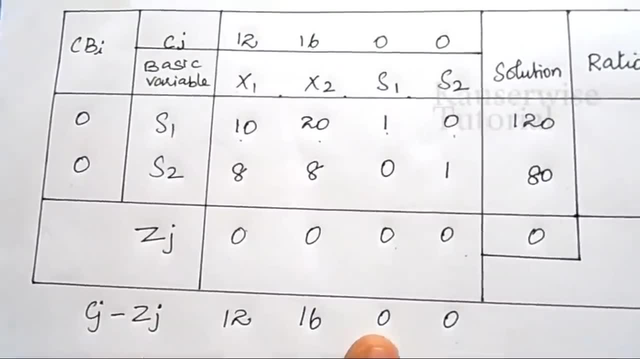 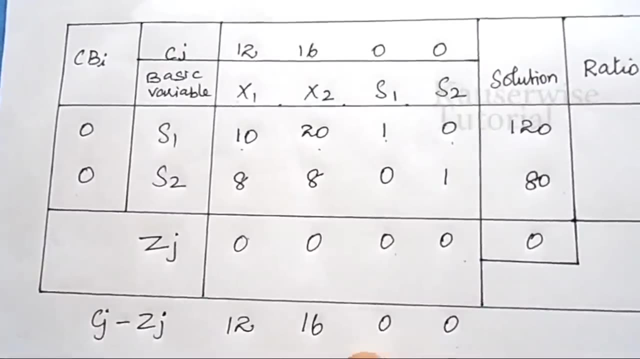 16.. third value: 0. fourth value: 0. see, this is the maximization problem. no, optimality condition is the final value, that is, cj. zj value should be 0 and less than 0, which means we need to get the negative value here. we have got positive values, no, so we did not reach the optimality, so we need 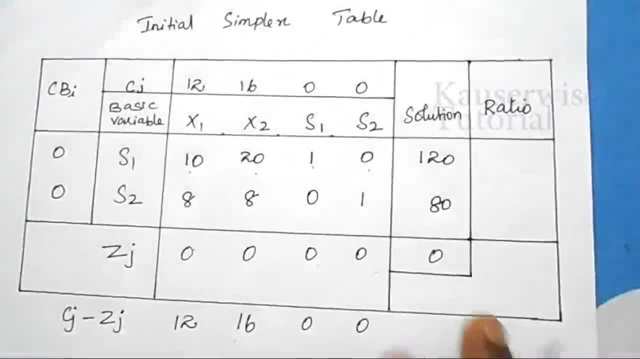 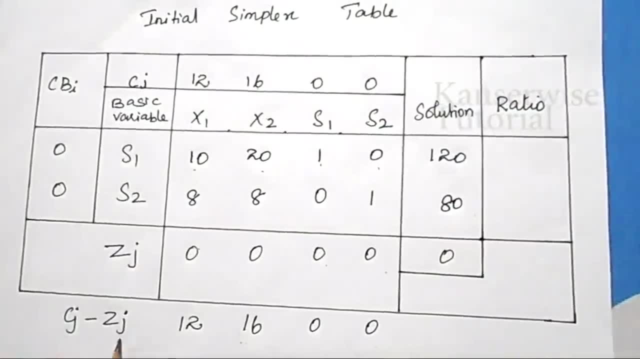 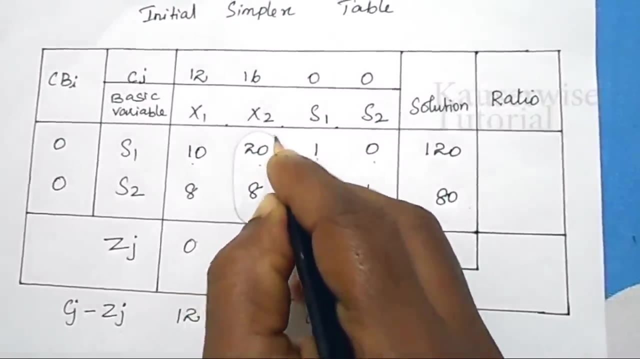 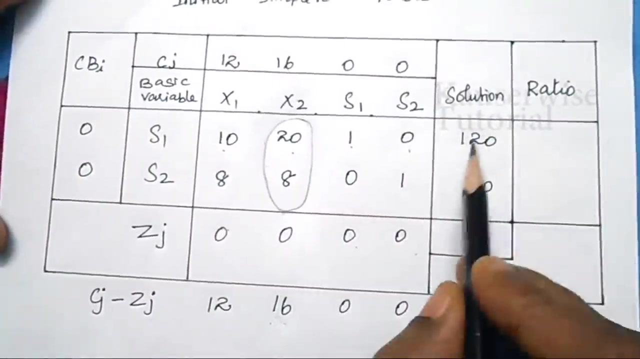 to proceed. further step to reach the optimality. in order to proceed further. first step is select the maximum value in the cj minus zj. c6, 16 is the maximum value. okay, so this column is called key column. after finding the key column, the next step is you need to find a ratio, that is, the ratio between solution column and key column. 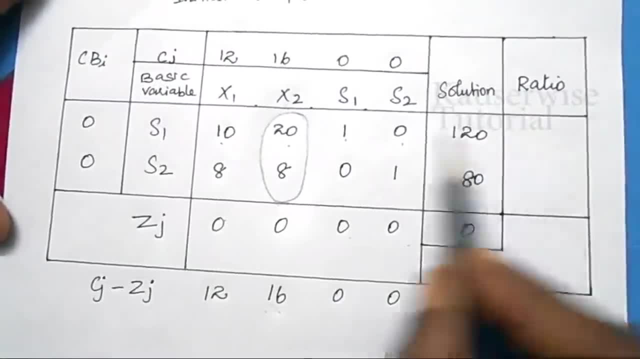 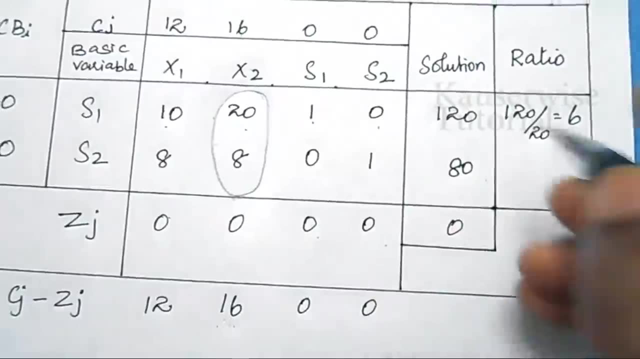 for the first row, solution is 120. no, so 120 divided by 20, you'll be getting ratio 120 divided by 26. in the same way, for second row, 80 divided by 8 is equal to 120 divided by 20. so this is the. 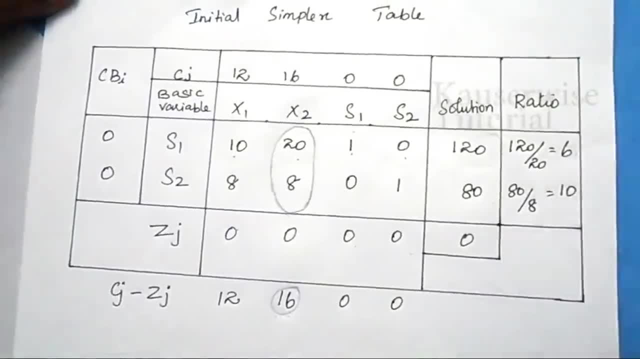 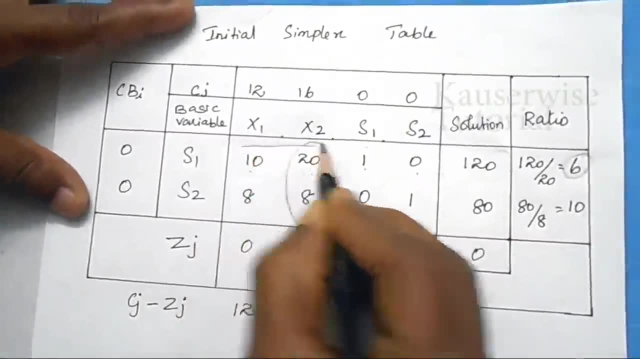 minimum value for second row: 80 divided by 20 is equal to 10. in order to find the key row, select the least value in the ratio column. here, 6 is the least value. that is minimum value. so this row, select this row. this row is called key row. this intersection point is called key element. this: 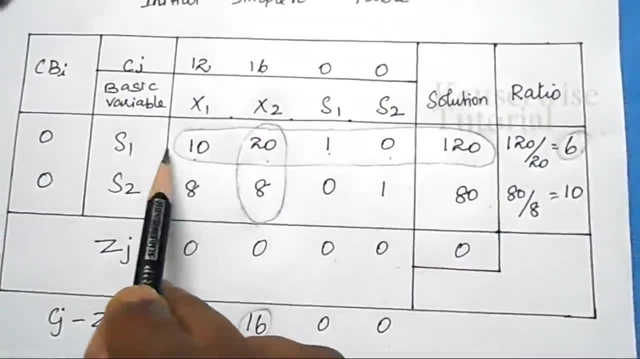 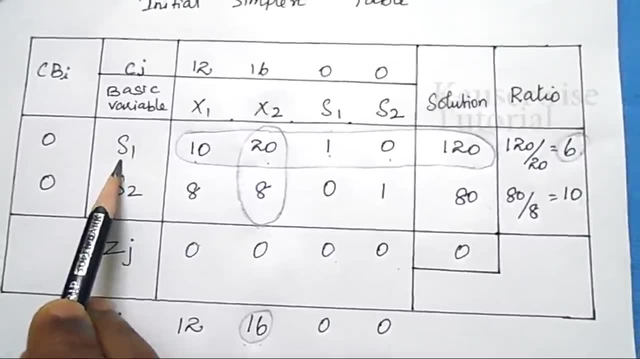 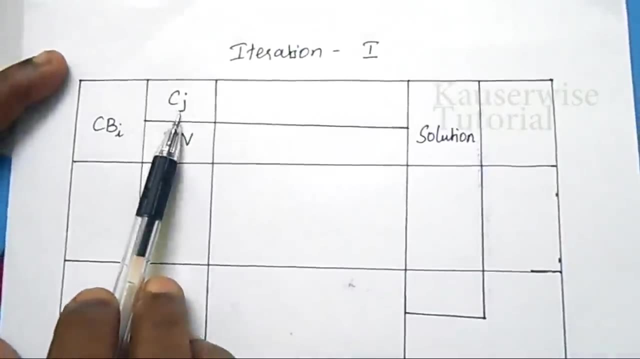 column is called key column. this row is called key row. here x2 is a entering variable, s1 is a leaving variable. now let us see how i am going to frame the first iteration. in the first iteration. first you need to write cj values and basic variables. 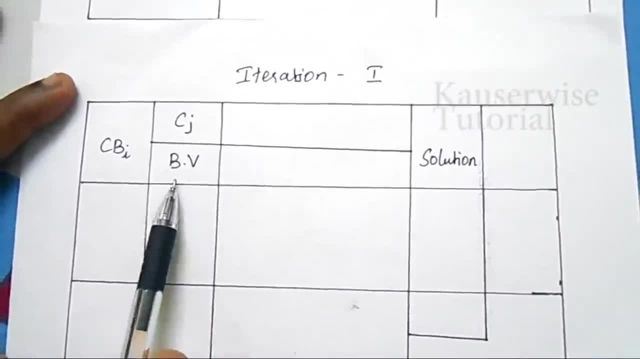 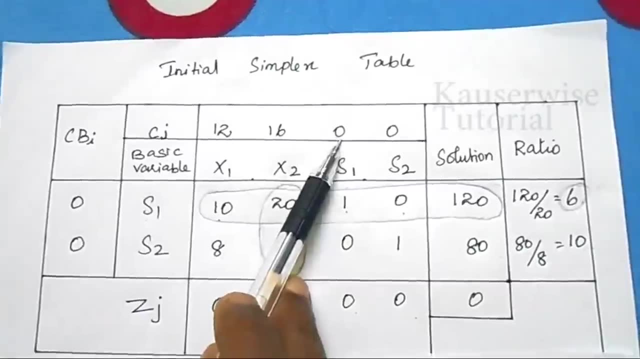 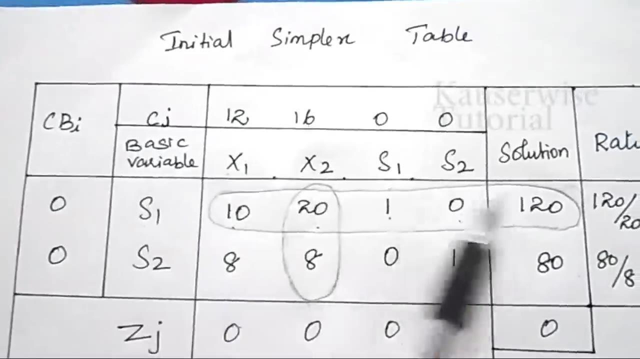 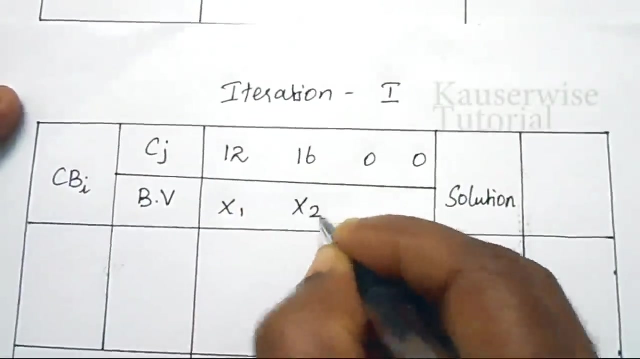 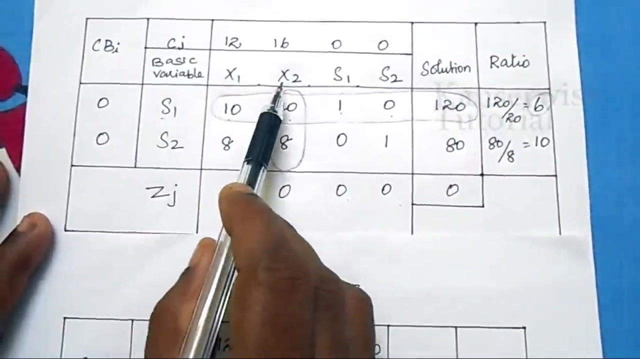 so there will be no changes in cj values and basic variables. just copy from the initial simplex table. cj is 12, 16, 0, 0, 12, 16, 0 and 0. basic variables are x1, x2, s1, s2. in the previous table we have found that s1 is a leaving variable and x2 is a entering variable. 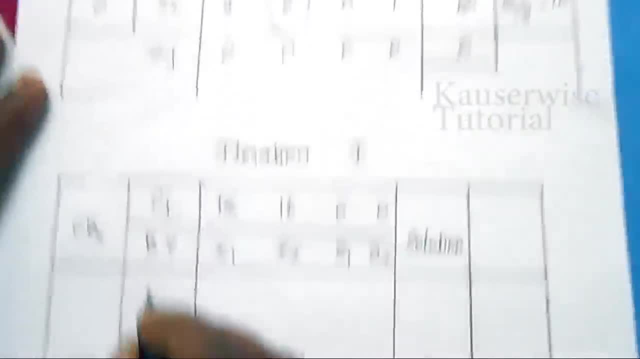 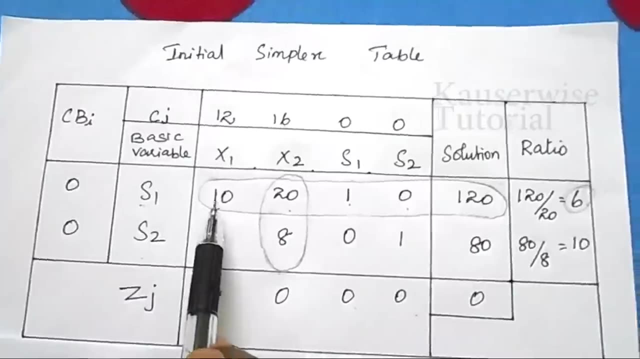 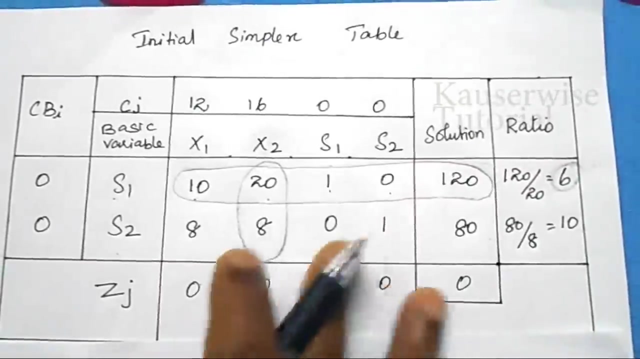 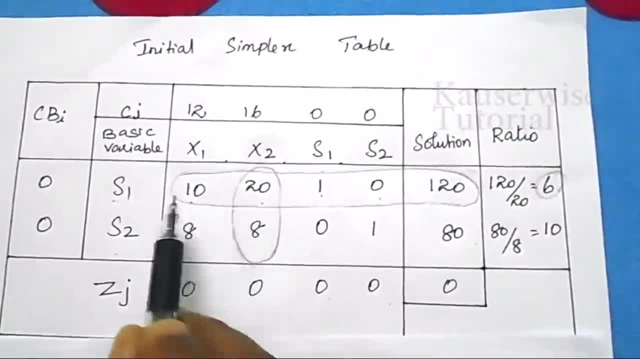 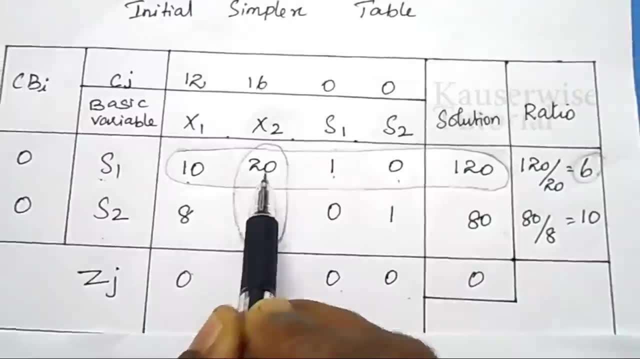 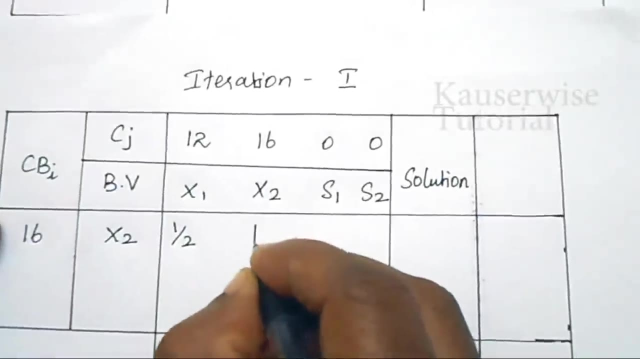 10 divided by key element. key element is 20. so 10 divided by 20 is equal to 1 by 2. second value: 20. old value is 20. key element also 20. no, so 20 divided by 20, 1 for this value. old value is 1. now you need to find the new value, 1 divided by 20. 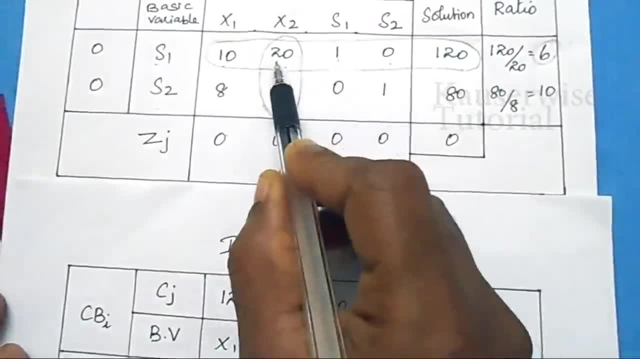 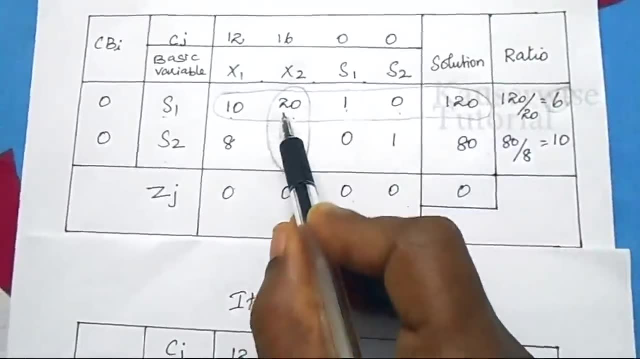 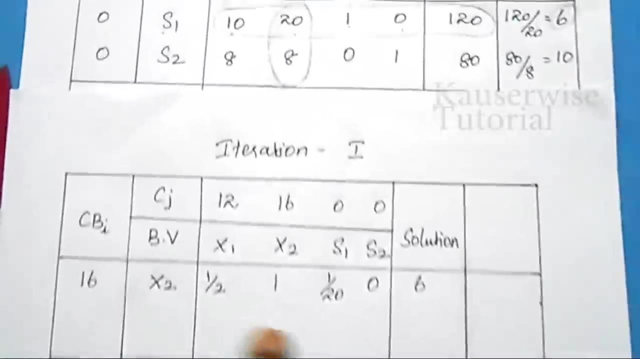 for this value, old value is 0: 0 divided by 20: 0. next one: 120, is old value. now for new value: 120 divided by 20: 6. we have got the values for first row. now you need to find the value for second row, that is s2. first write the basic. 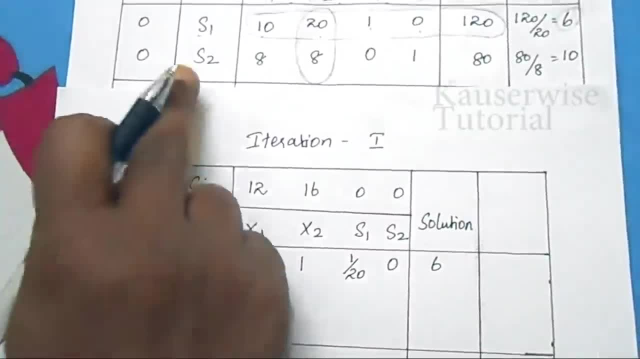 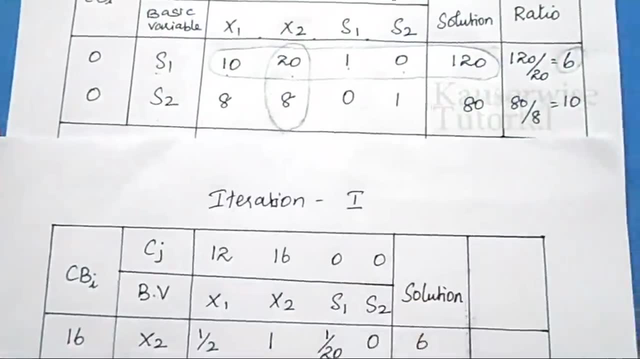 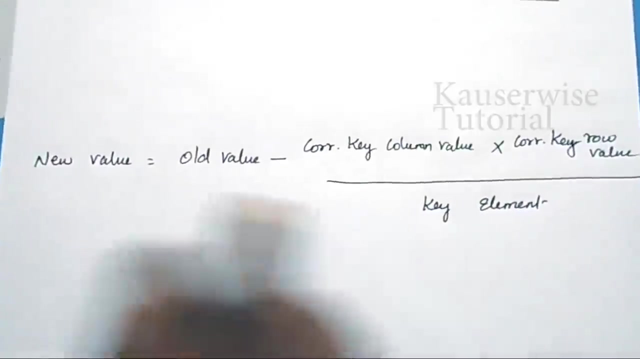 variable, that is s2, right as it is. what is the value cost? 0. write 0 here for all other elements. in order to find the new value, you need to apply a simple formula. so there is a formula to find out the new value. this is the formula to find the new value, that is, old value minus corresponding. 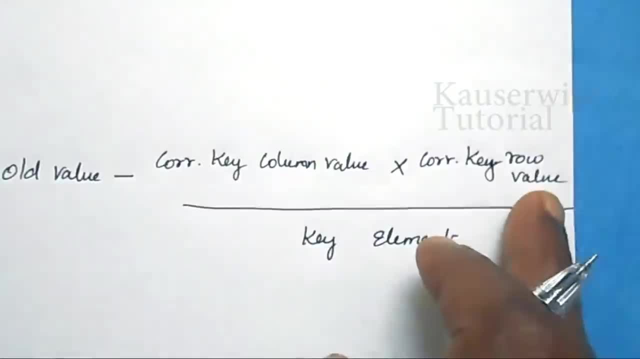 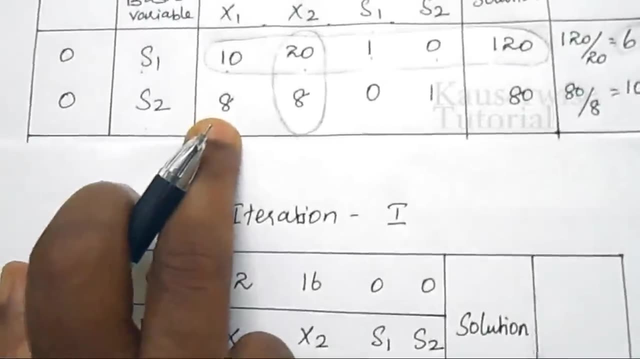 key column value into corresponding key row value divided by key element. so let me explain. look at the first value. old value is 8. okay, write 8 here. old value is 8, minus corresponding key column value, into corresponding key row value divided by key element. so let me. 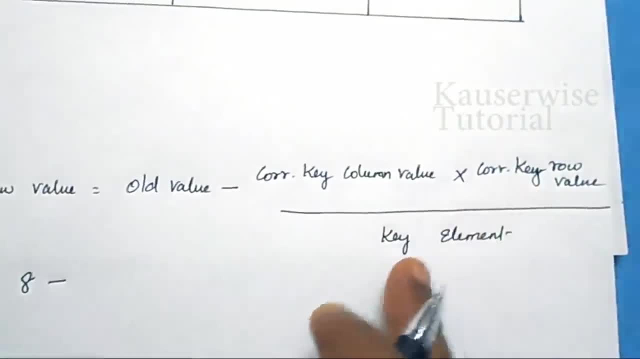 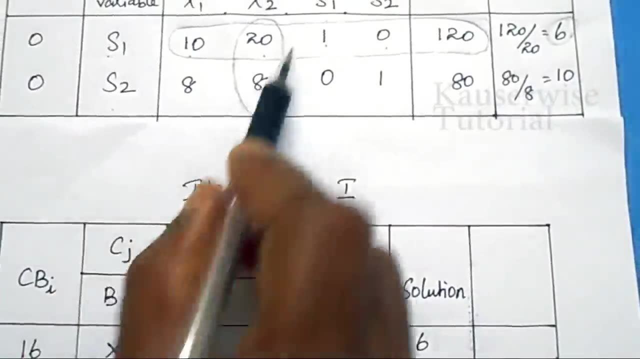 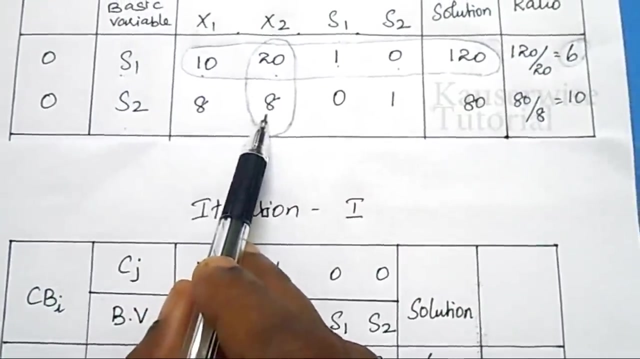 the difference between the corresponding key column value and key row value divided by key element. see here: the old value is 8. no, so corresponding column value is 8. this is the key column. this one is key row. okay, here the corresponding key column value is 8. corresponding key row value is 10. 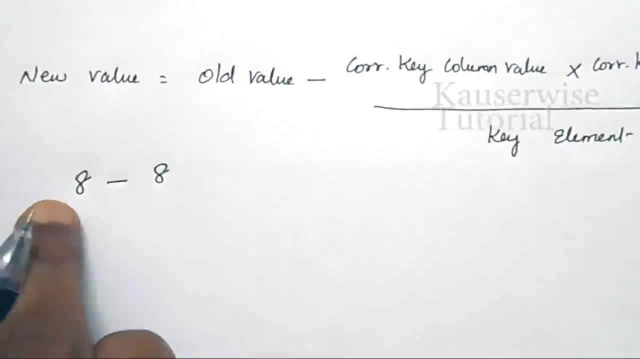 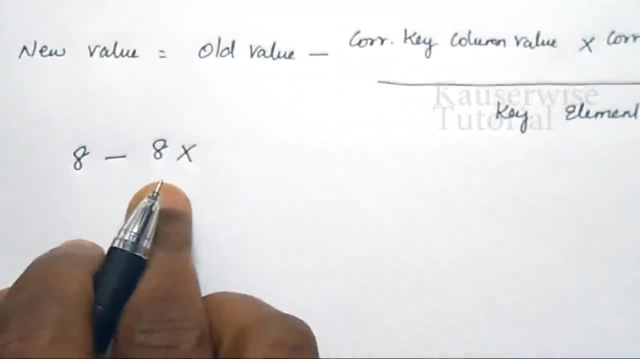 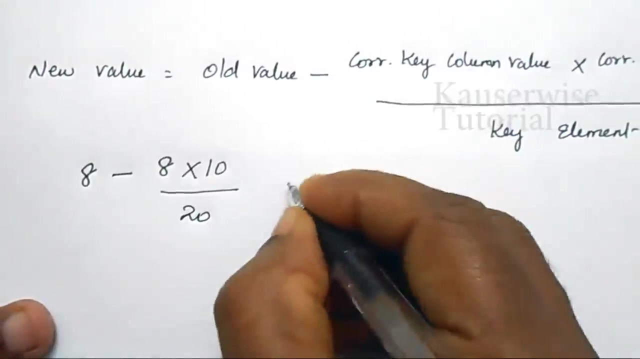 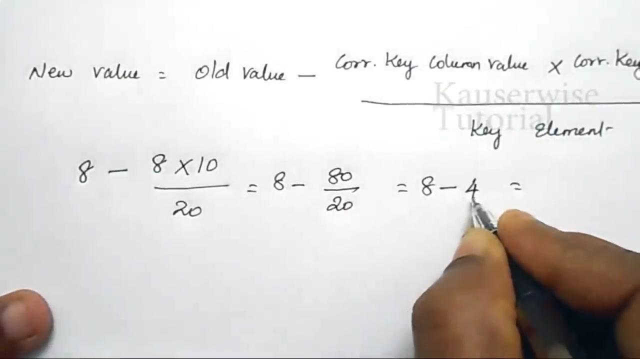 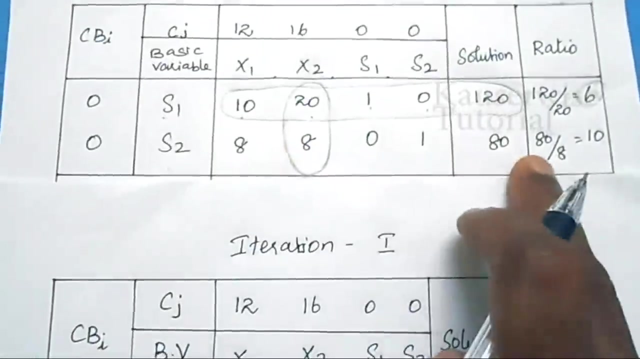 divided by key element is 20. old value: 8 minus corresponding key column value. also 8 into corresponding key row value is 10. divided by key element is 20. 8 into 10, 80, 8 minus 80 divided by 20. so 8 minus 4 is equal to 4. write 4 here in the same way. find the value for all other values also. 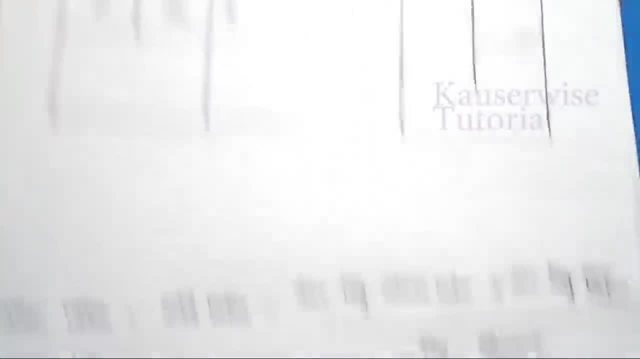 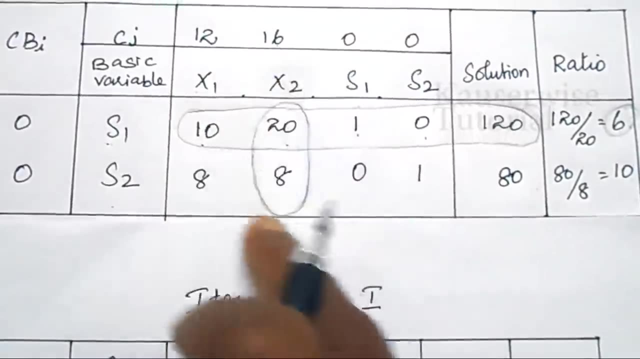 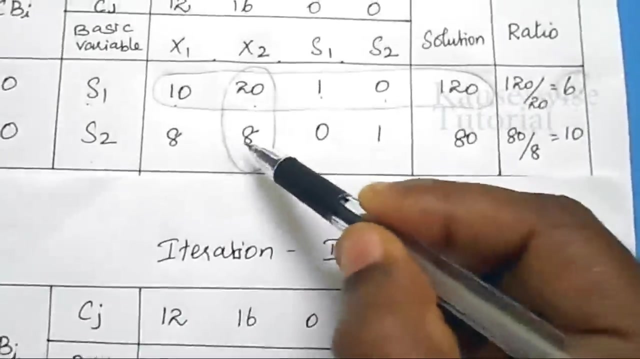 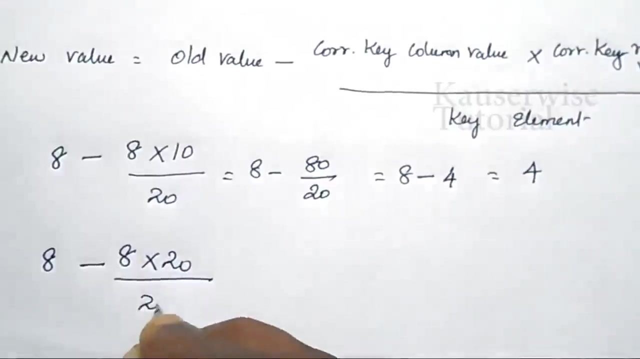 the next one is 8. old value is 8. old value: 8 minus corresponding key column value. key column is this: so key column is same thing, only 8. 8 into corresponding row value. corresponding row value is 20. okay, 20 divided by so the key element is common for all the values. so old value is 8. 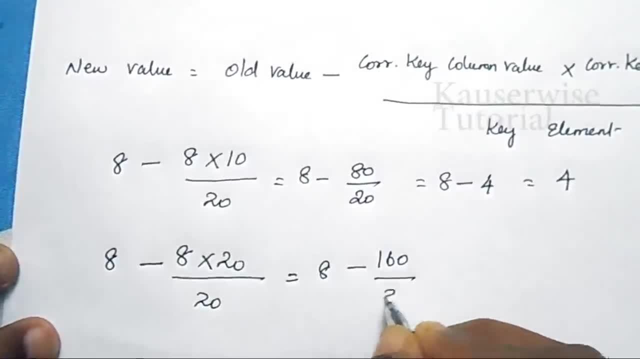 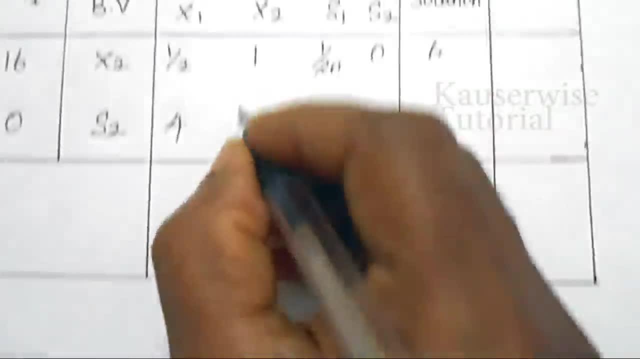 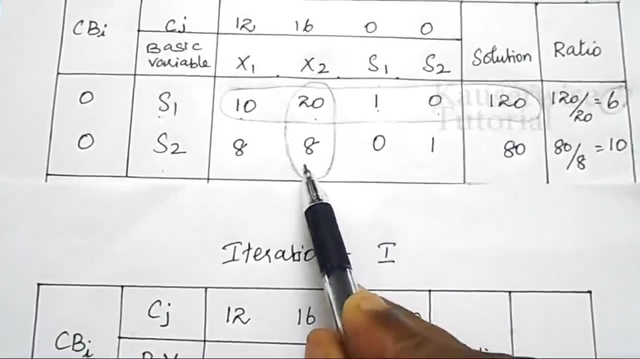 8, 8, 8 minus 8 into 20, 160 divided by 20. so 8 minus 8 is equal to 0. new value is 0: 0. in the same way, for the next value, old value is 0. corresponding column value: 8 into corresponding: 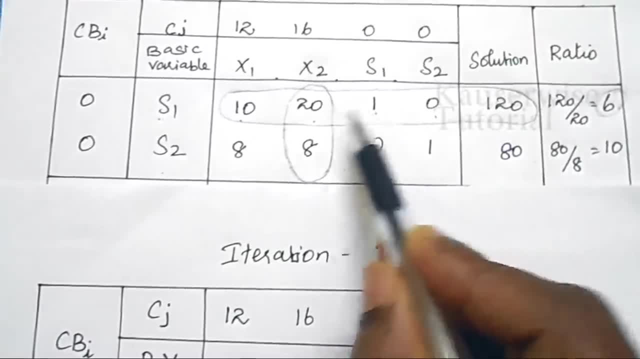 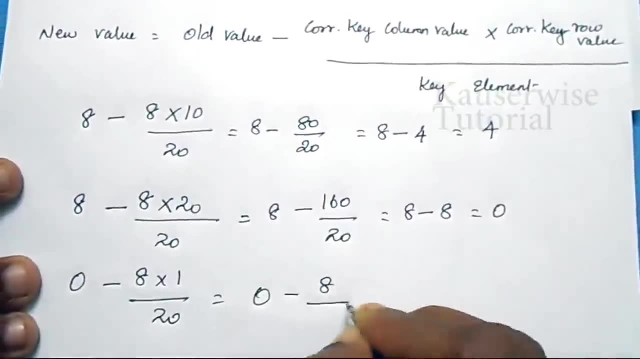 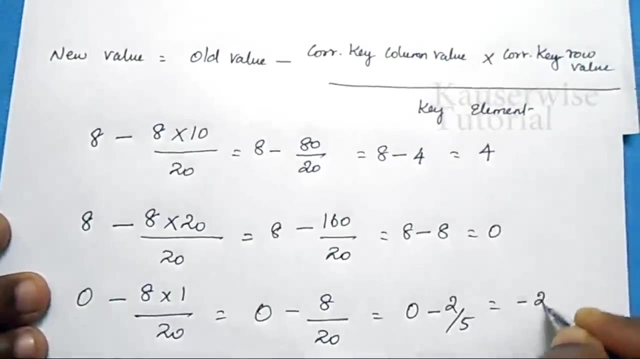 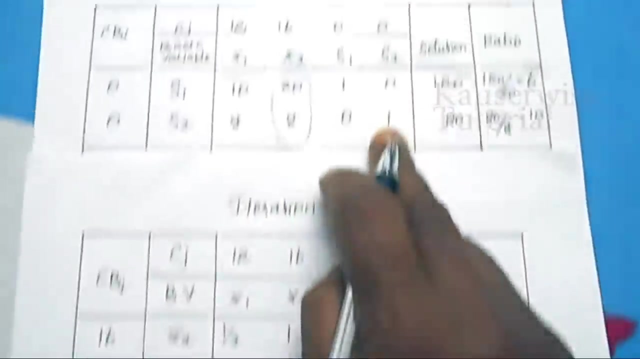 row value 1 divided by corresponding key element, 20, into value. divided by 20 so 0 minus 8. divided by 20 so 0 minus 2 by 5, so minus 2 by 5, minus 2 by 5. in the same way for the next value, old value. 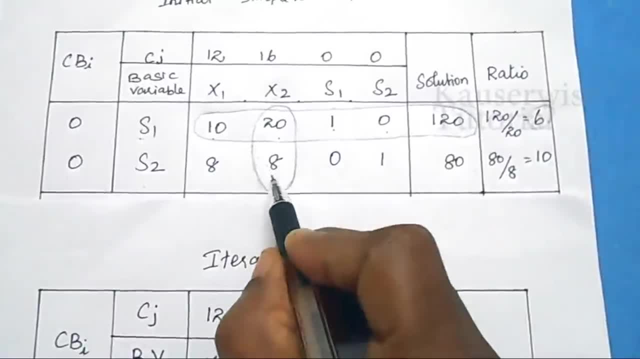 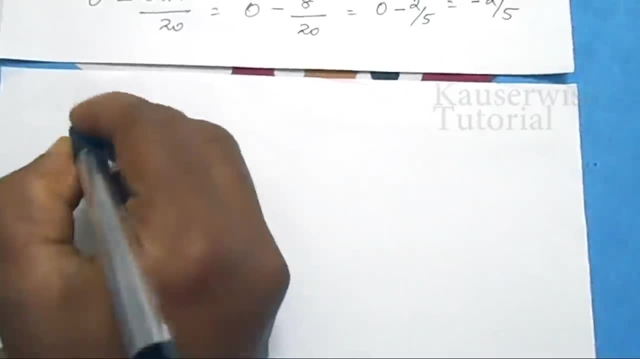 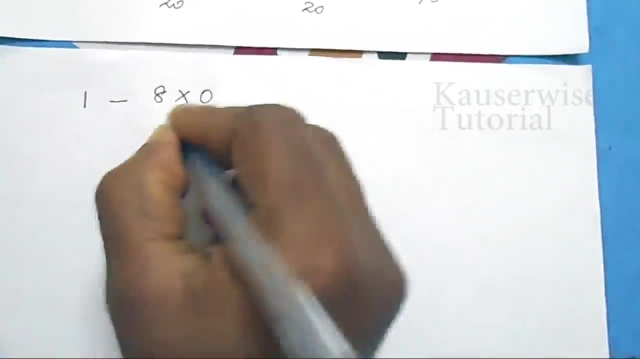 1 minus corresponding column value 8 into corresponding row. value 0 divided by corresponding key element 20. old value 1 minus corresponding column value 8 into corresponding row. value 0 divided by corresponding key element 20, so 1 minus 8 into. 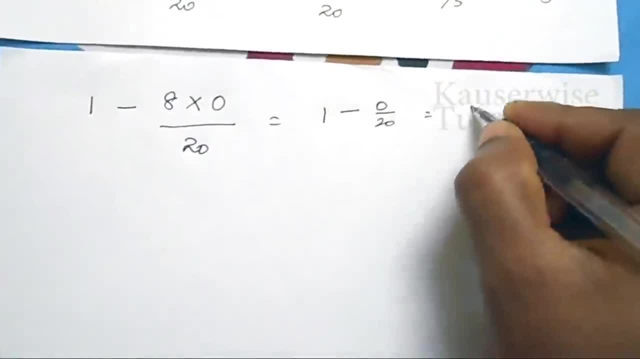 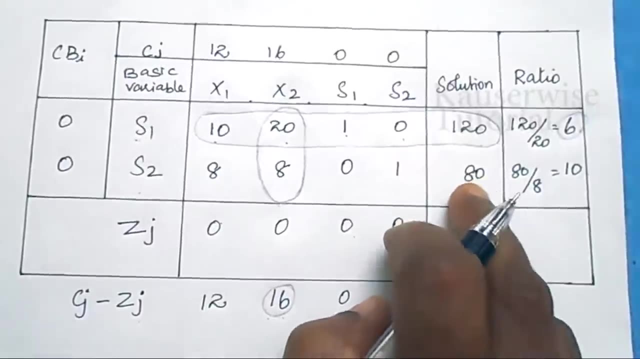 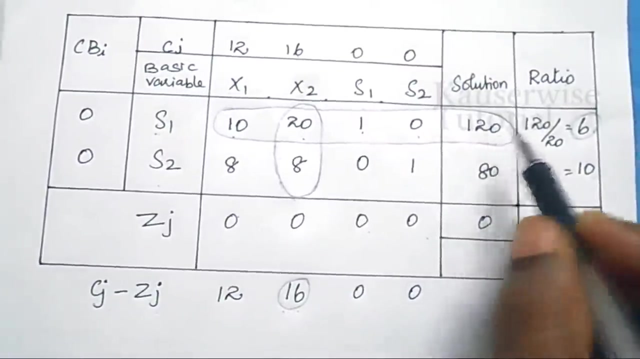 0. 0 so 0 minus 20. 0 only so 1 so 1. in the same way for the next value, old value is 80. no so 80 minus corresponding column value. 8 into corresponding row value: 120 divided by corresponding key element: 20 old value: 80 minus corresponding. 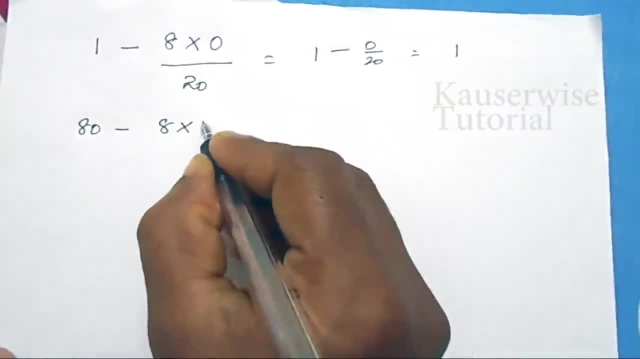 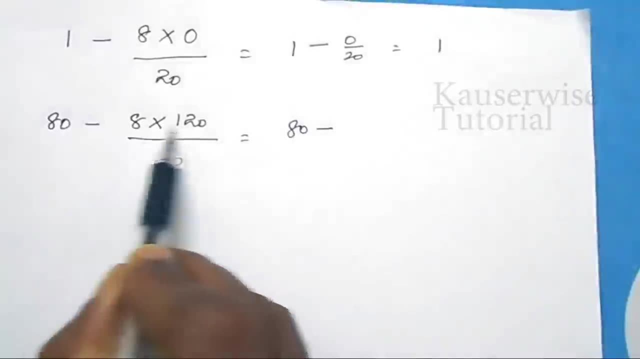 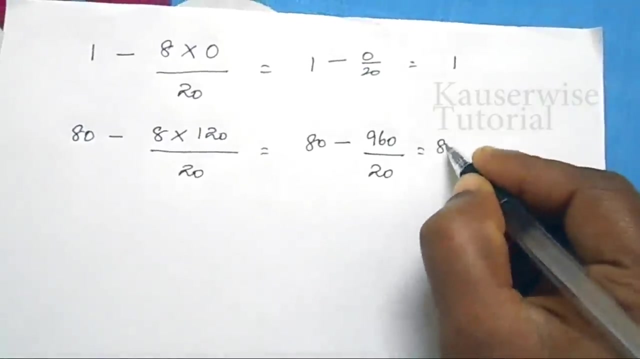 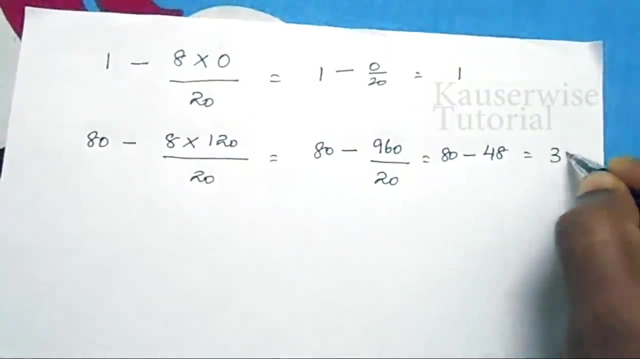 column value 8 into corresponding row. value 120 divided by key element: 20, so 80 minus 8, into 20. 960 divided by 20, so 80 minus 960 divided by 20: 48, final answer is 32. 32 is the new value. so now, 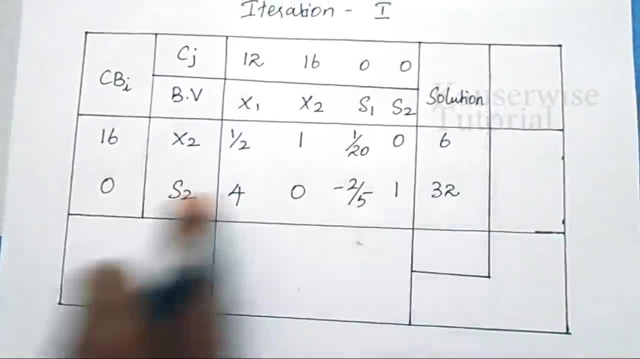 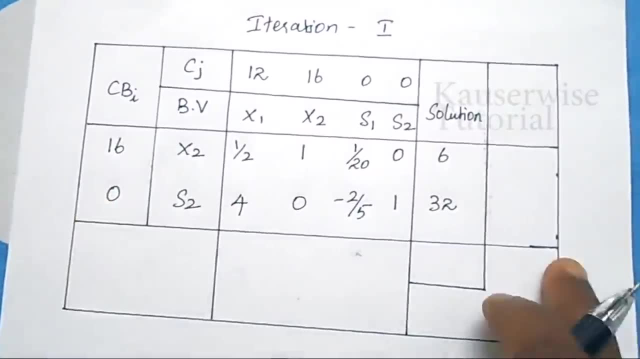 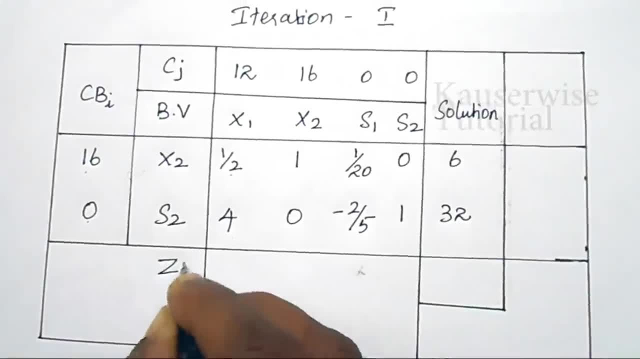 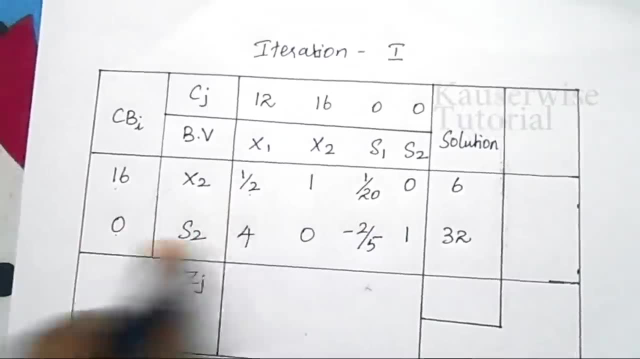 second row. now you need to find zj. okay, the formula for zj is: multiply cbi value into x value, each element plus in row value 0 into 4. that is, 16 into 1 by 2 plus 0 into 4. what is the? 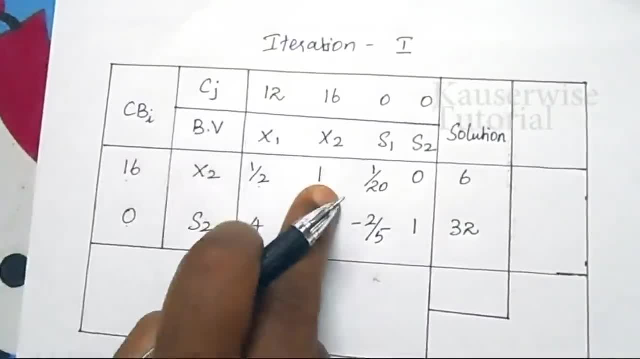 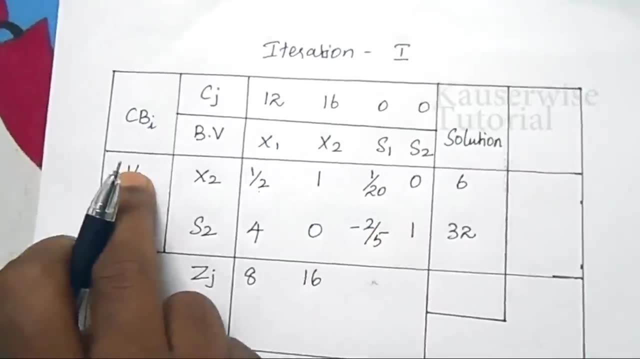 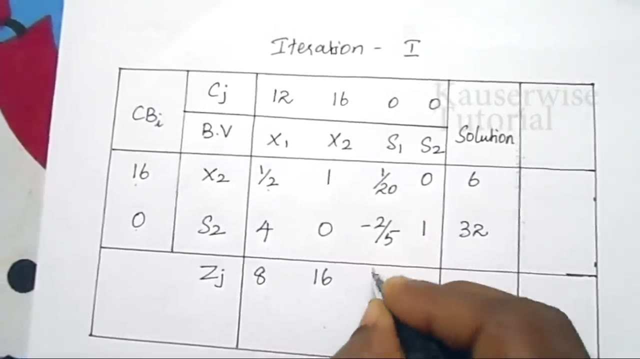 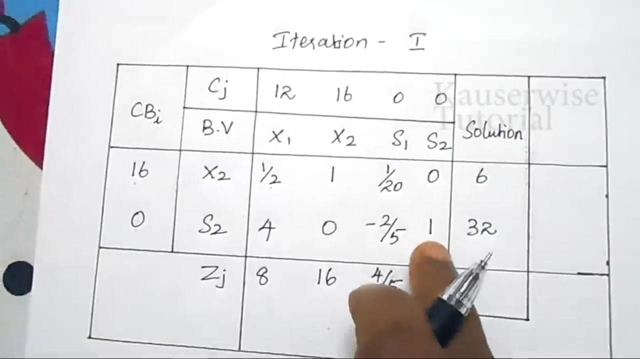 value 8. for the second value: 16 into 1 plus 0 into 0, 16 for the third value: 16 into 1 by 20 plus 0 into minus 2 by 5. answer is 4 by 5. for the next value: 16 into 0 plus 0 into 1, 0, so after: 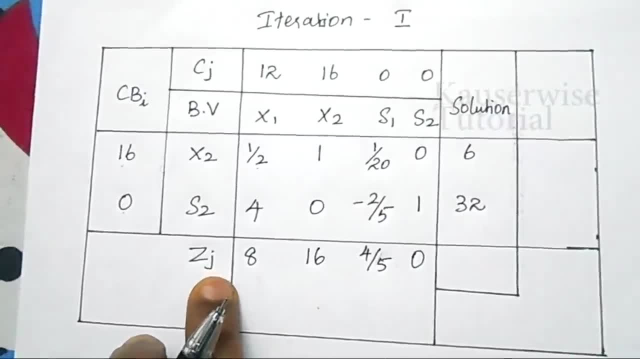 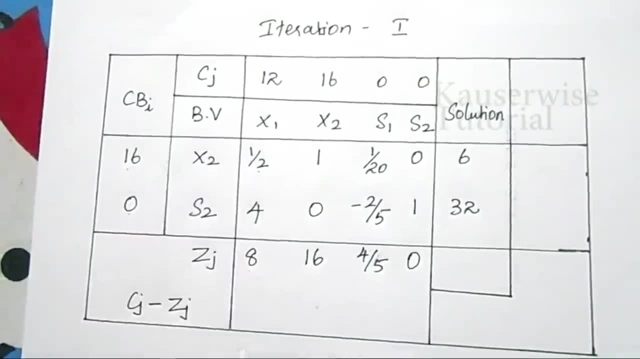 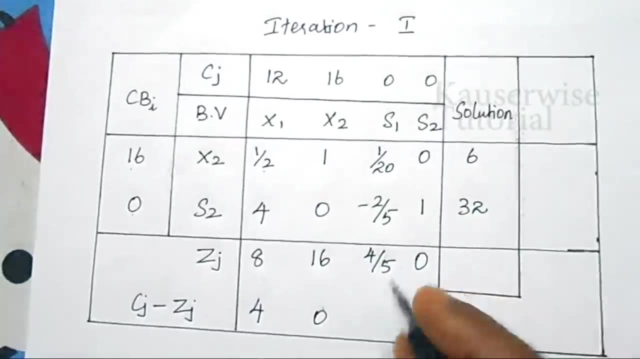 finding zj, then you need to compare cbi value into x value and then you need to compare cbi value into zj value with zj value. that is cj minus zj. that is 12 minus 8, 4, 16 minus 16, 0, 0 minus 4 by 5 minus. 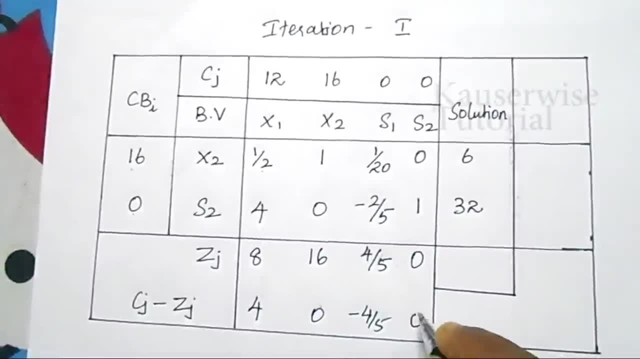 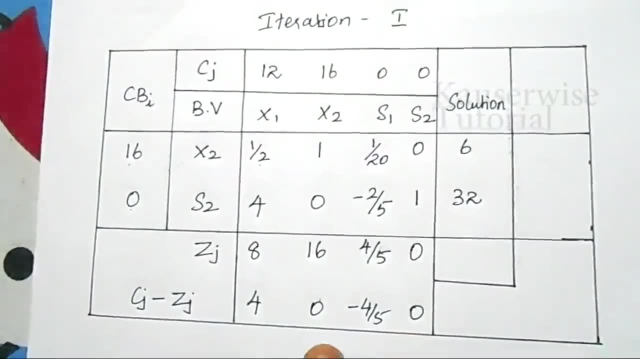 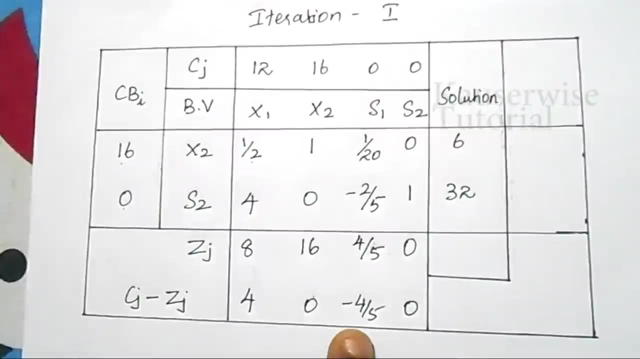 4 by 5, 0 minus 0, 0. so what is the optimality condition? cj minus zj must be 0 and less than 0, which means 0 or negative value. here we have got 4, 0 minus 4 by 5 and 0. here we have one positive value. so we have to proceed further. 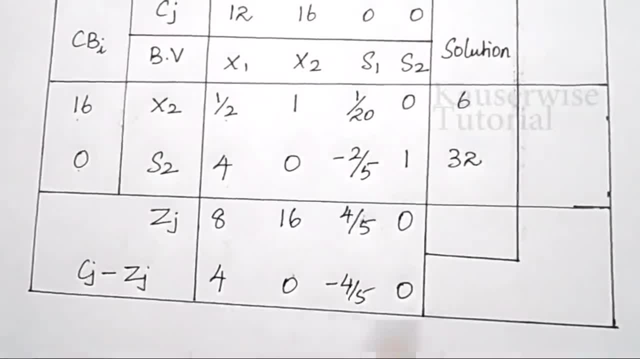 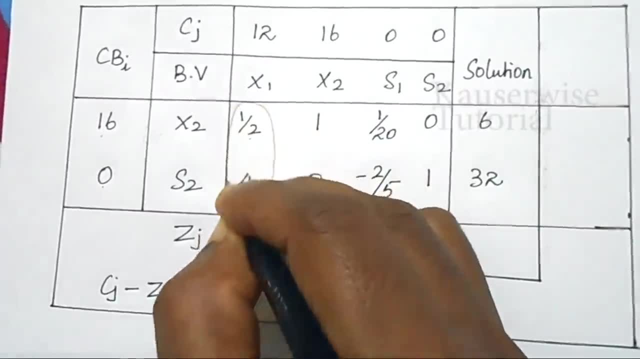 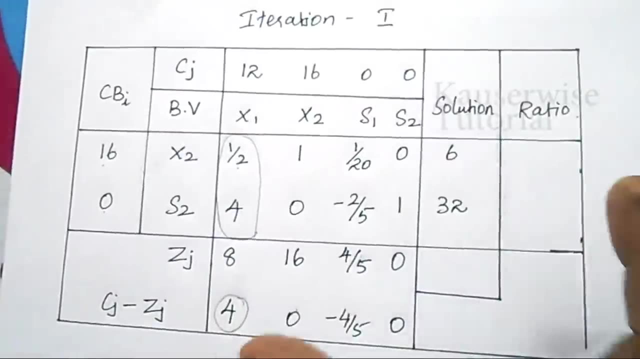 in order to proceed further, select the maximum positive value. here, 4 is the maximum positive value, so select this column. this column is a key column. okay, after finding the key column, then you need to find the ratio. you need to find the ratio with solution value and key. 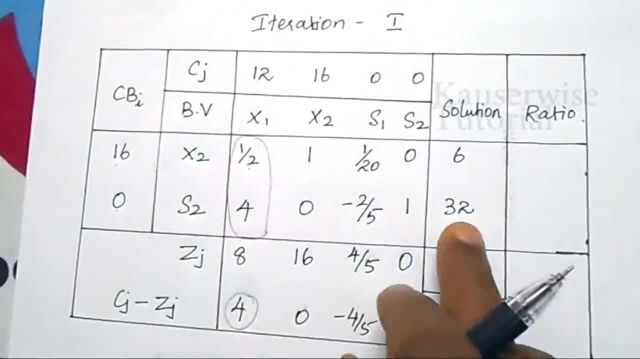 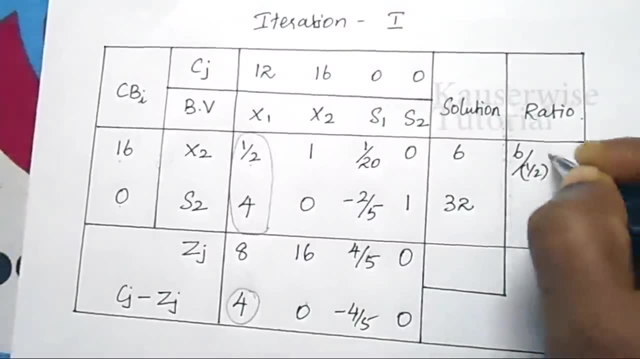 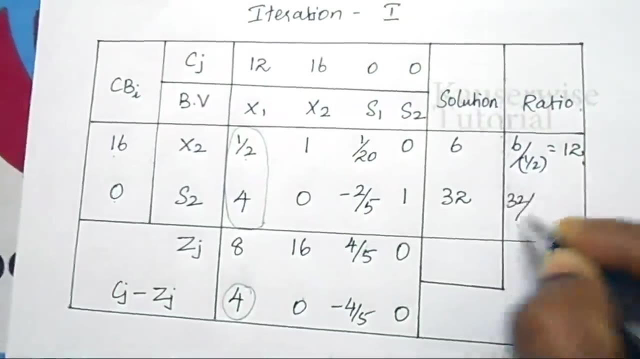 column value. that is, 6 divided by 1 by 2 and 32 divided by 4. for the first row, 6 divided by 1 by 2. what is answer? 12. in the same way for the second row, the solution is 32. no, 32 divided by key column. 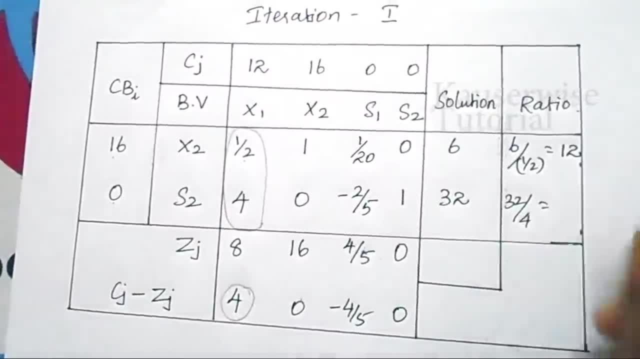 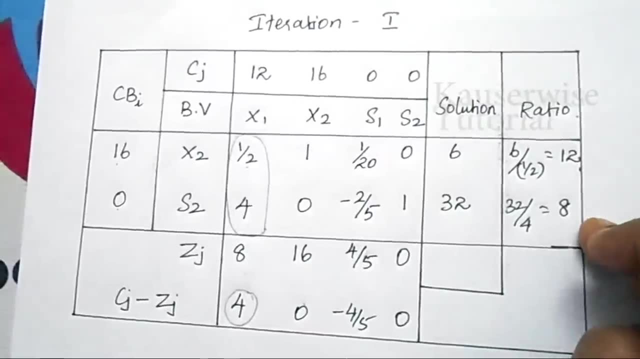 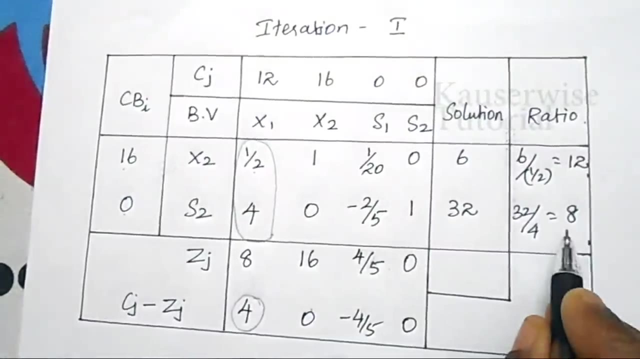 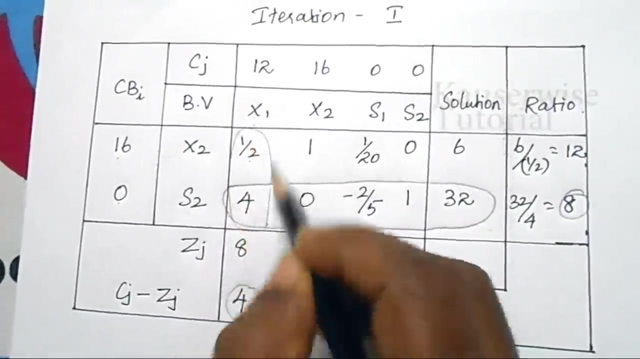 value is 4- 4. what is answer? 8. okay, so now we have got two ratios. now we need to select the key row. so, in order to select the key row, we need to find the least value, that is, minimum value. so which one is least value? 8 is the least value. no, select this row. this row is called key row. this column is called: 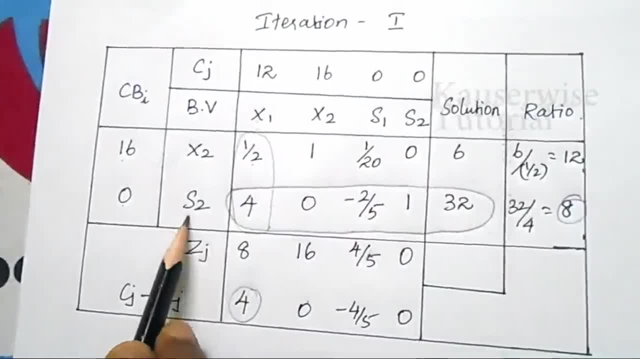 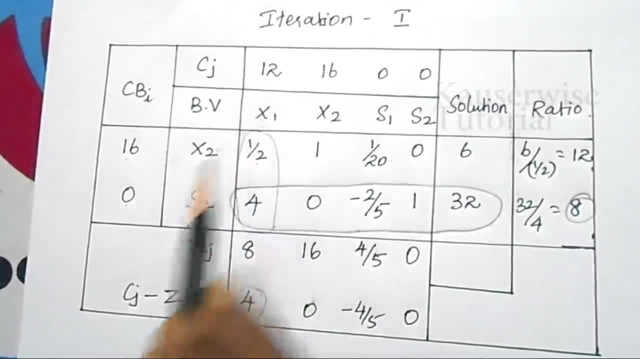 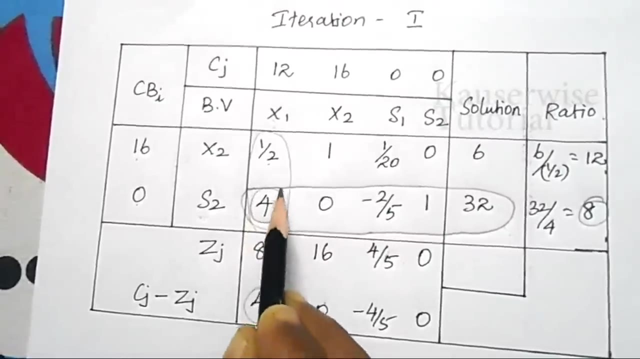 key column. see. the row variable is s2. no, the row variable will be leaving variable. the column variable will be entering variable. so x1 is a entering variable, s2 is a leaving variable. the intersect point is called key element. here 4 is the key element. so with this you need to proceed further. so now you need to find the. 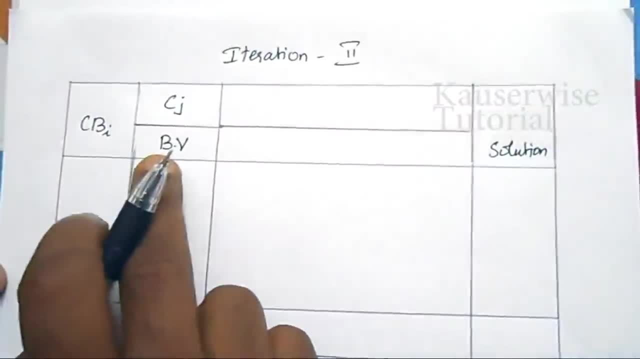 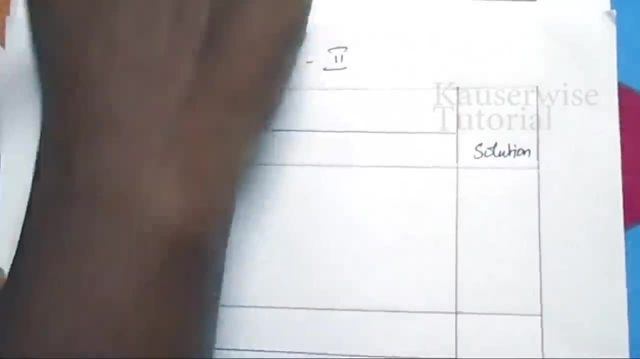 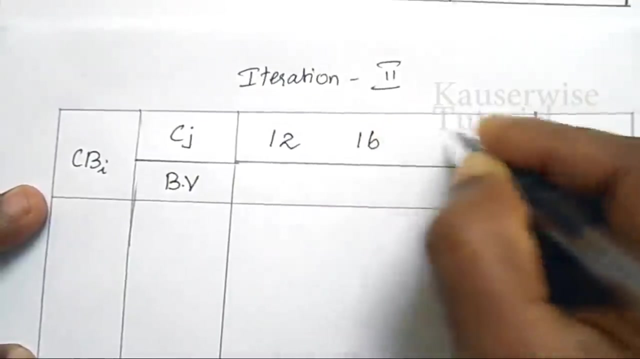 second iteration. in the second iteration write the basic variables and cj values. so there will be no changes in this. you can write the same thing which is there in the first iteration: cj values: 12, 16, 0 and 0, 12, 16, 0 and 0. basic variables are x1, x2, s1 and s2. 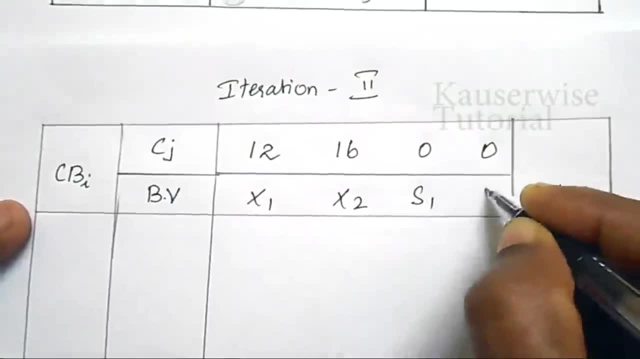 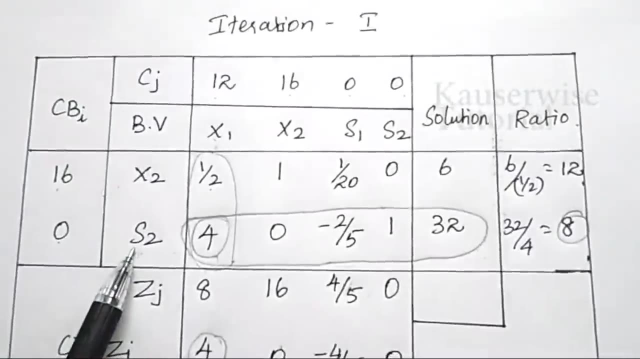 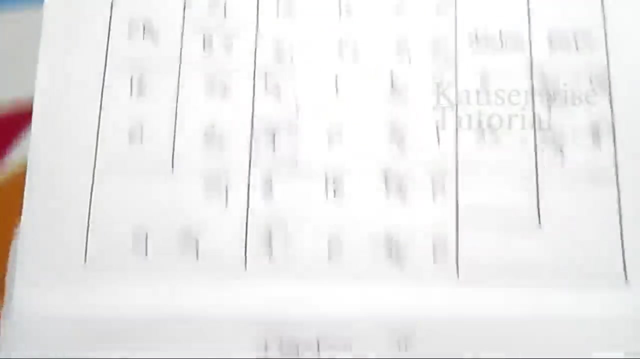 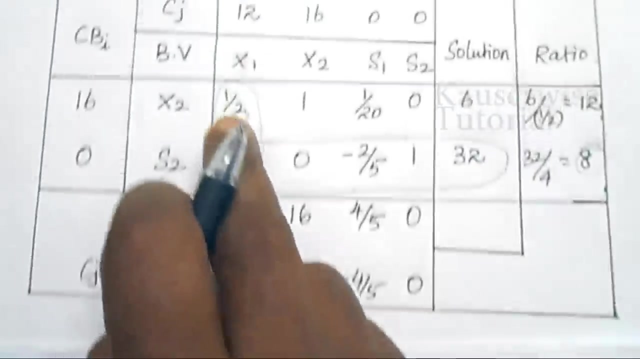 and s2. okay, in the basic variable column there are two variables, are there no here? x2 is a leaving variable, x1 is a entering variable. in the second iteration, write the same thing as it is x2. x2 cost is 16: 16. okay, now you have to write the second one, that is: 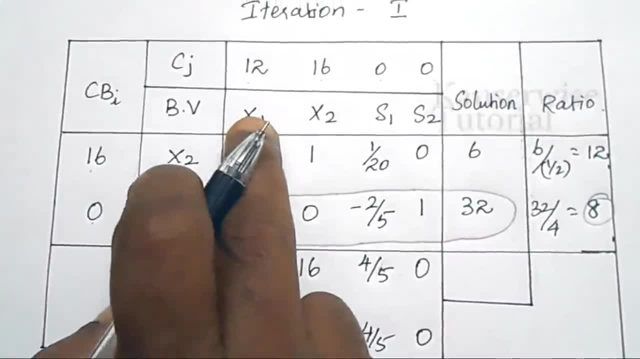 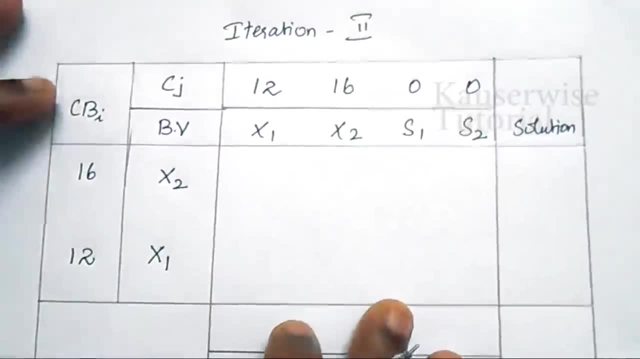 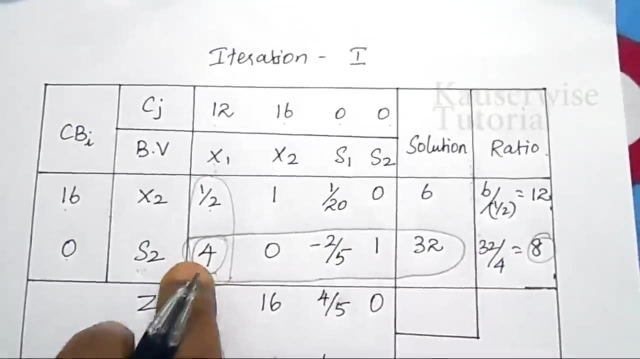 s2 is a leaving variable. entering variable is x2 and s2 is a leaving variable, so x2 is a leaving variable, x1. so instead of s2 you have to write x1 with the value. okay, now this is the key rono for new value. just divide the key element with the old value. 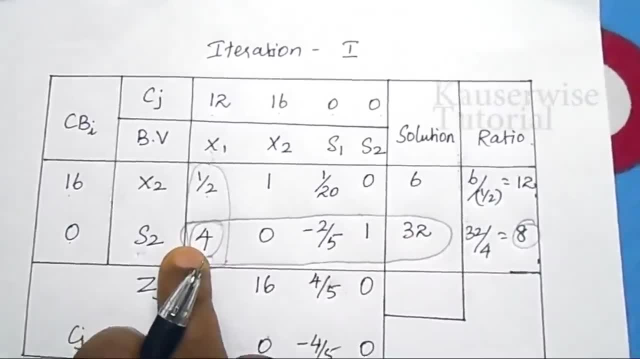 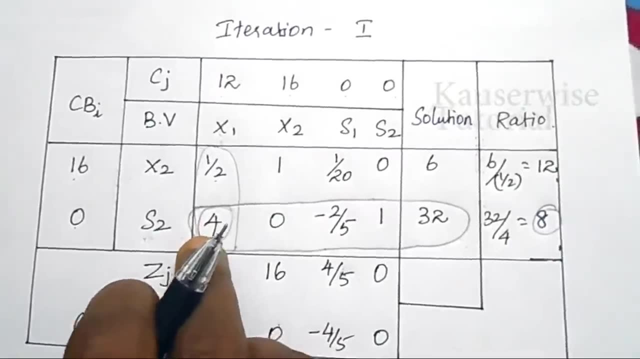 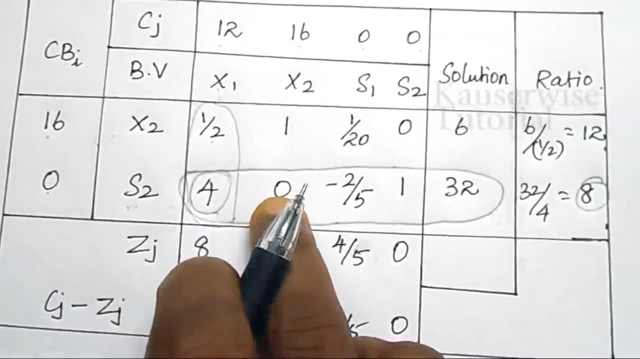 in order to find the new value in the second iteration. for the first value is old value. is 4 divided by key element. also same thing, only 4. so 4 divided by 4, 1, 1. second value: old value, 0, 0 divided by key element. 4, 0 divided by 4: 0. 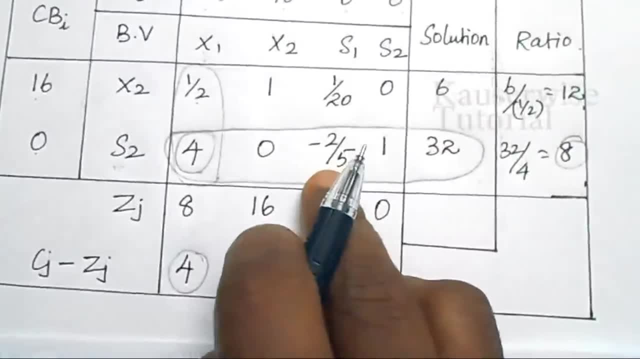 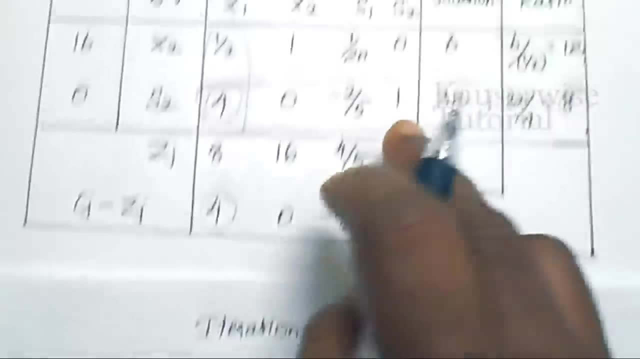 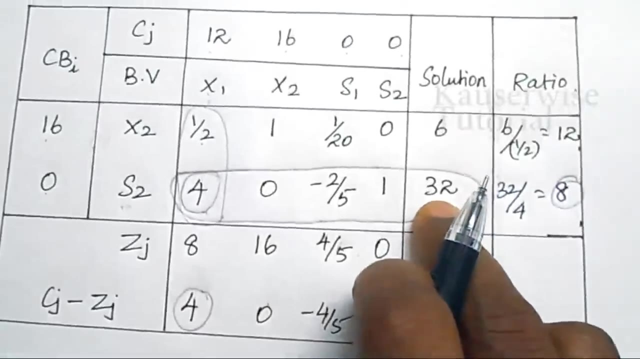 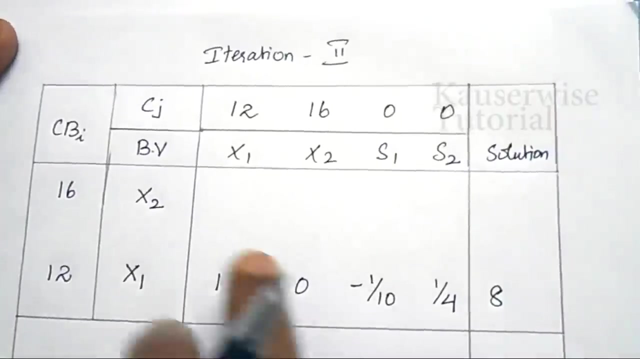 next value: minus 2 by 5 divided by 4. minus 1 by 10, next 1 divided by 4, then 32 divided by 4: 8. here we have got the new value for the second row, and now you need to find the value for first row. look. 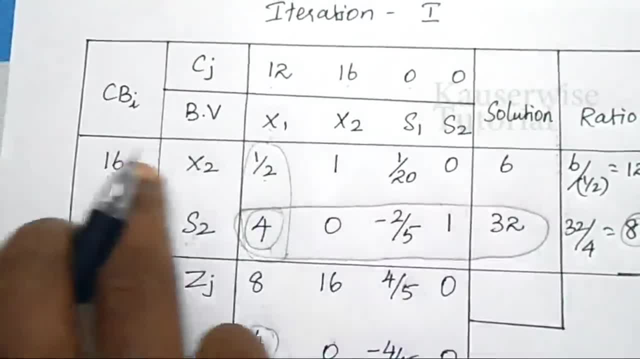 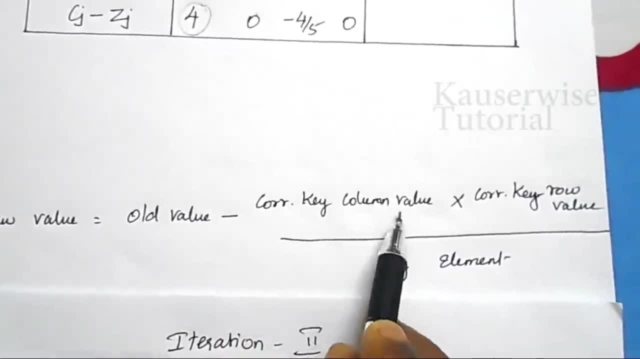 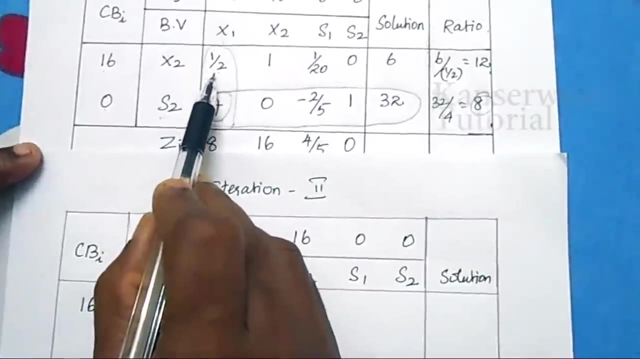 at the first iteration. here you need to apply the formula. what is the formula for these values? that is, new value is equal to old value minus corresponding key column value into corresponding key row value divided by key element. let us see: the old value is 1 by 2 the corresponding key. 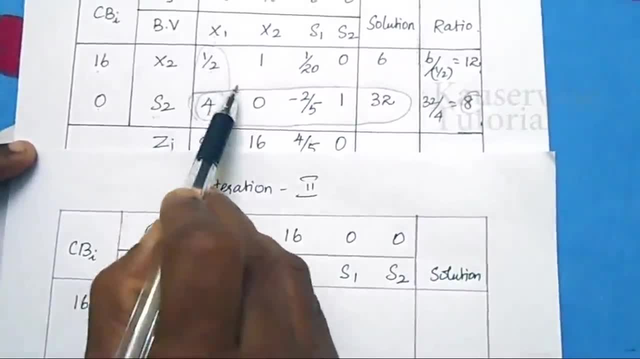 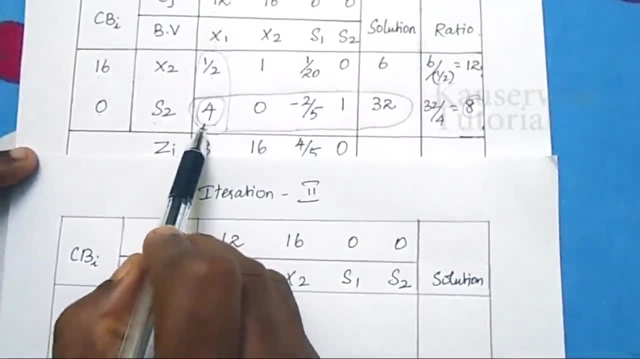 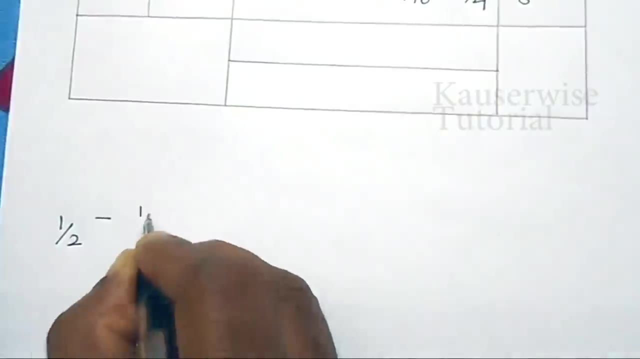 column value. also same thing, only 1 by 2 into corresponding row value. row values: 4 divided by corresponding key element. that is, key element is common for all the value. that is 4 old value 1 by 2 minus corresponding column value, also 1 by 2, into. 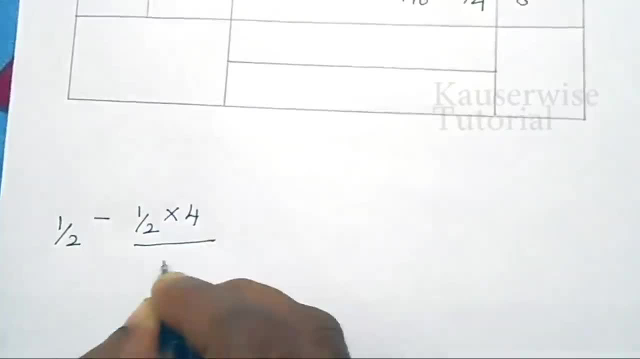 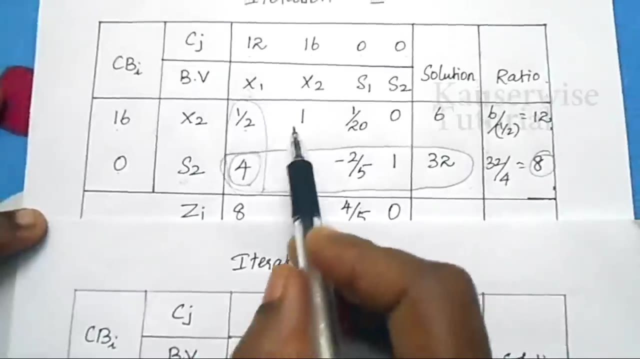 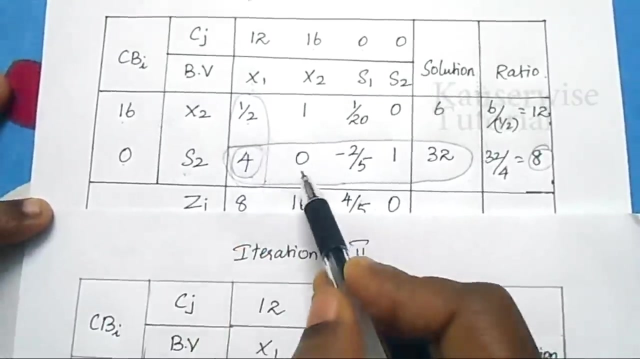 corresponding row value 4 divided by key element 4, the answer is 0: 0 for the second one: old value 1 minus corresponding column value 1 by 2 into corresponding row. value 0 divided by key element 4. old value 1 minus corresponding column value 1 by 2 into corresponding row. 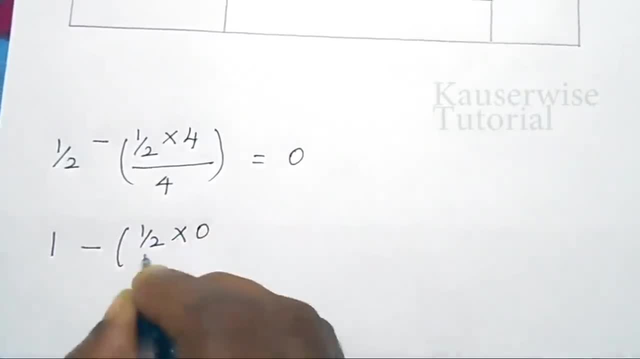 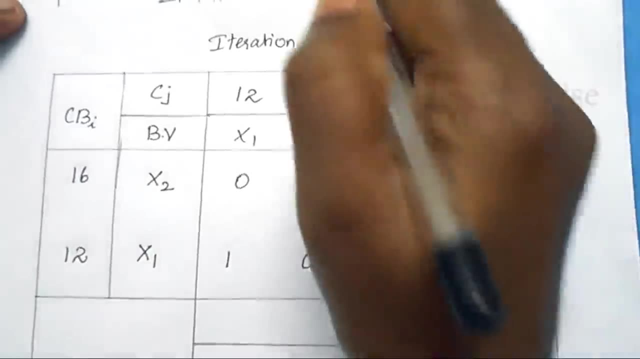 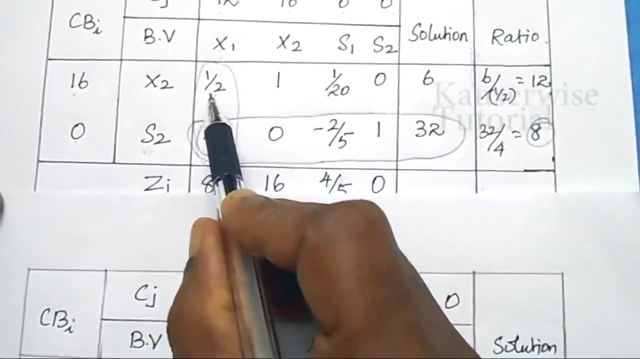 value 0 divided by key element 4, the answer is one. for the next value, old value is 1 by 20, minus corresponding column value 1 by 2, into corresponding row value 0, K element shell and one sub value 0, the value of queied 2 is. addこれは три значies if to the key elementeloat stronger value 7.. ett этого걸성. 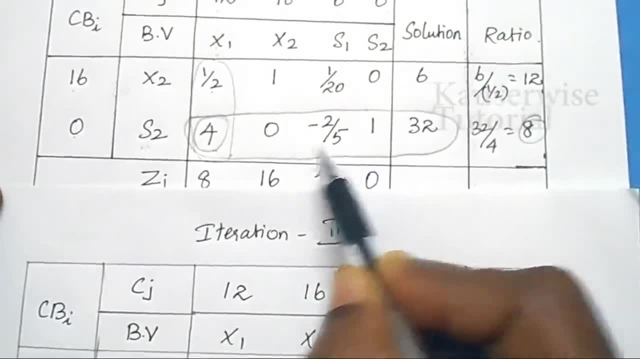 pkechia's value 0 is 0 in the backom show. here is a koll deinen value of the problem: preparation action: corresponding row value minus 2 by 5 divided by key element: 4.. Old value: 1 by 20, minus corresponding. 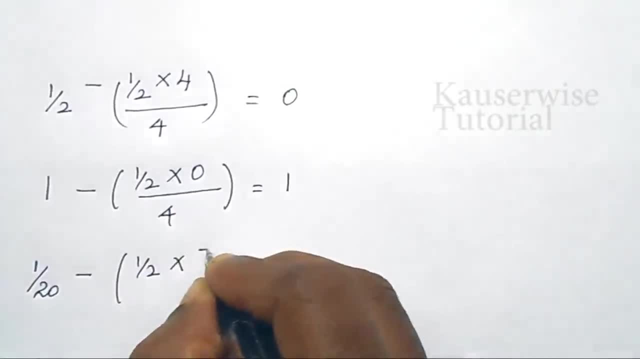 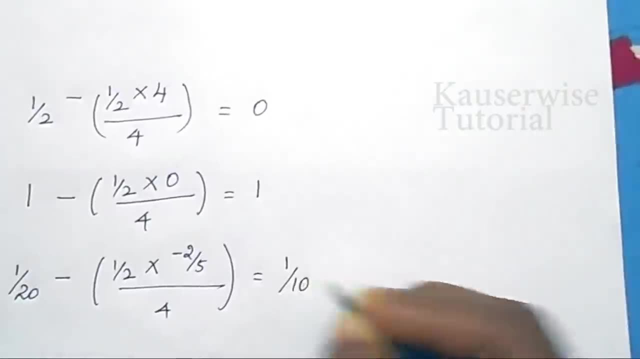 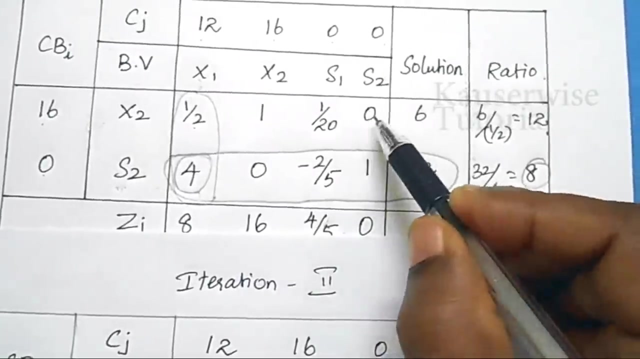 column value 1 by 2 into corresponding row value minus 2 by 5 divided by key element 4.. The answer is 1 by 10.. For the next value, old value 0 minus corresponding column value 1 by 2 into: 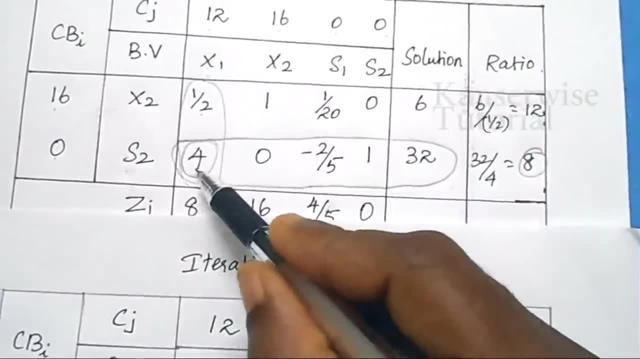 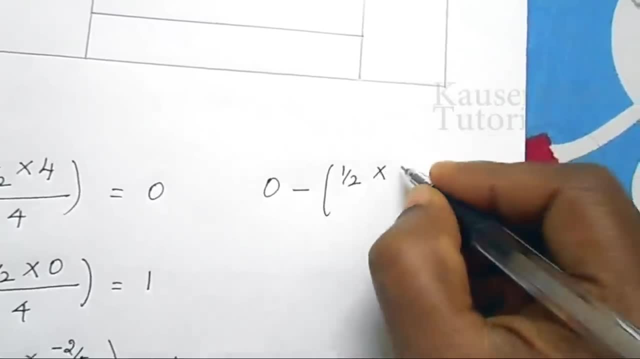 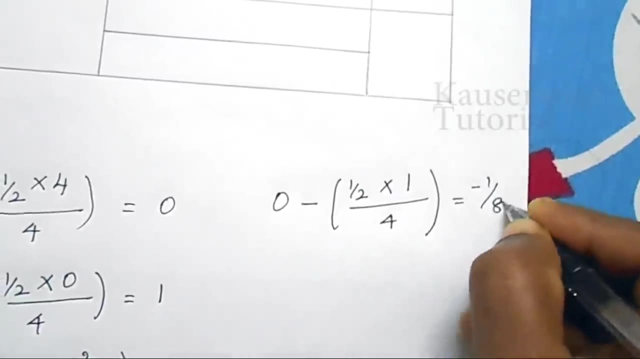 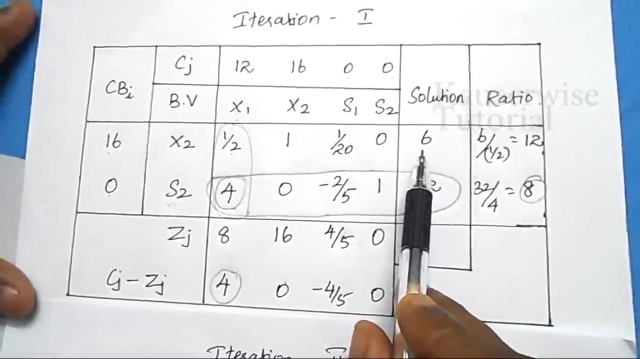 corresponding key row, value 1 divided by key element 4.. Old value 0 minus corresponding column value 1 by 2 into corresponding row value 1 divided by key element 4.. Answer is minus 1 by 8.. For the next value, old value 6 minus corresponding key column value 1 by 2. 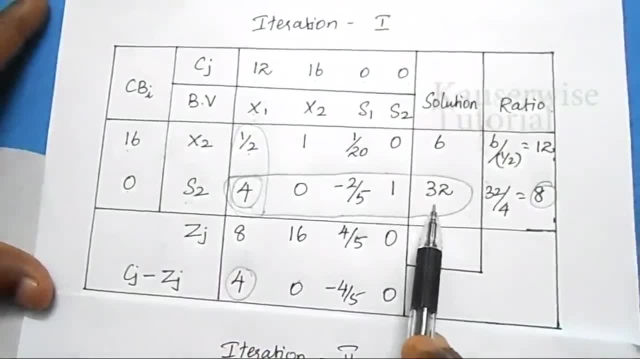 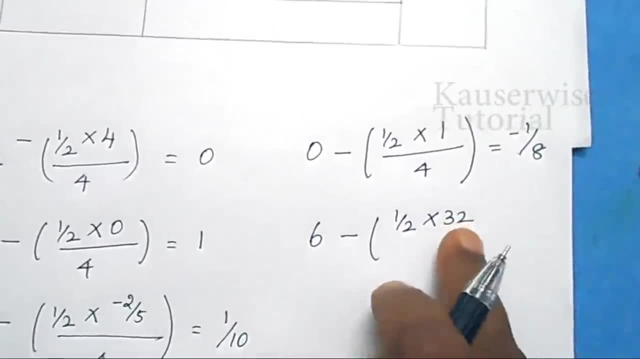 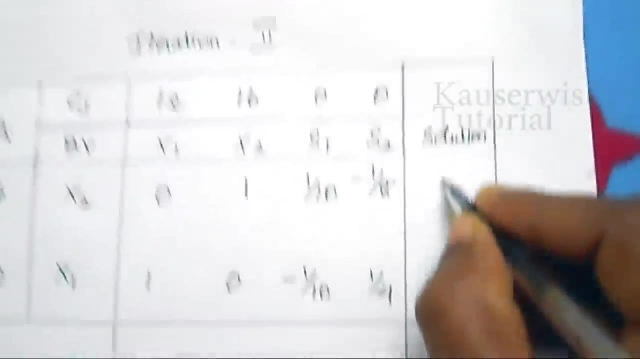 into corresponding row value 32, divided by key element 4.. Old value: 6 minus corresponding column value 1 by 2 into corresponding row value 32, divided by key element 4.. The answer is: 2.. After finding the new values, we will find the new values. We will find the new values. 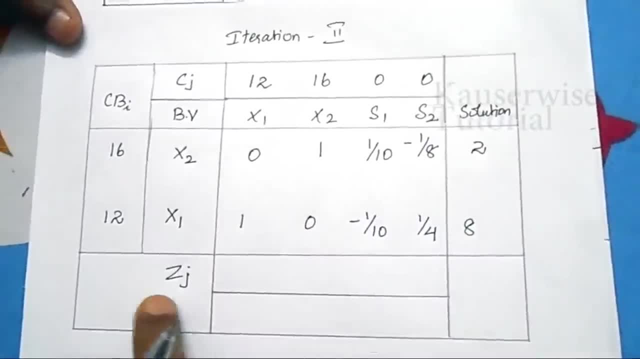 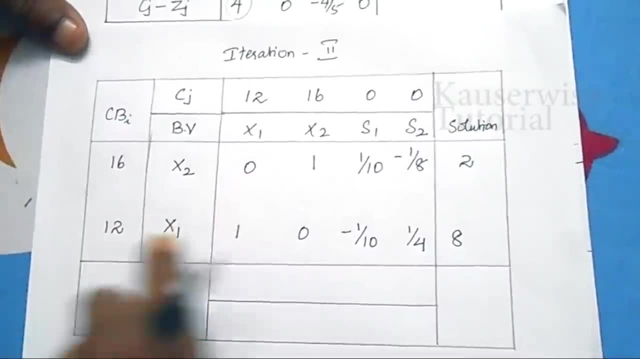 For two rows. now you need to find Zj. To find out Zj, take cost into each element. That is 16 into 0 plus 12 into 1.. What is the value? 16 into 0, 0 plus 12 into 1, 12..